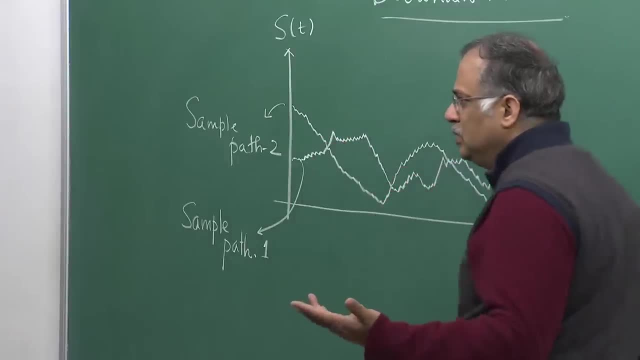 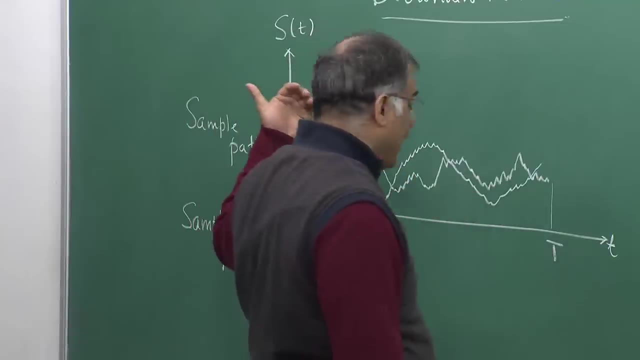 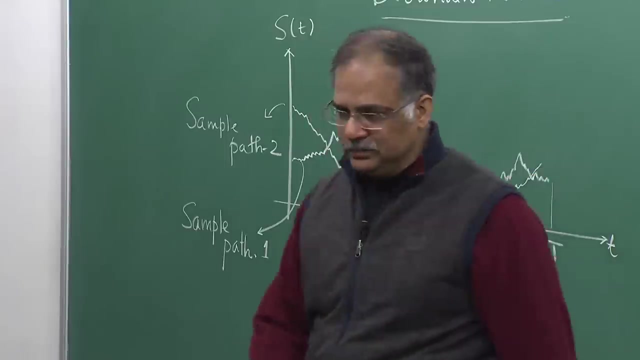 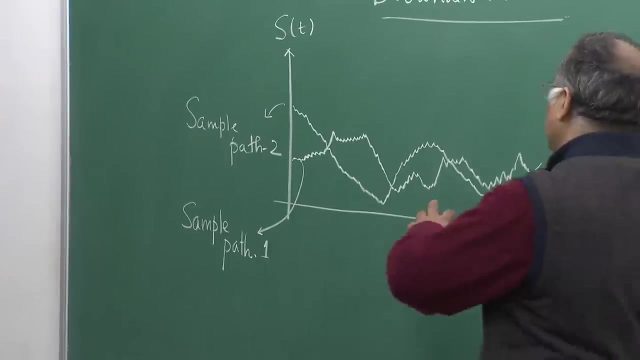 zigzagging paths. What way to model it? Is there any mathematical way to say that? or can I construct the stochastic process whose sample paths are represented in this form? Let us do. to do that, We need to study what is called Brownian motion. Brownian motion is a type of stochastic process. 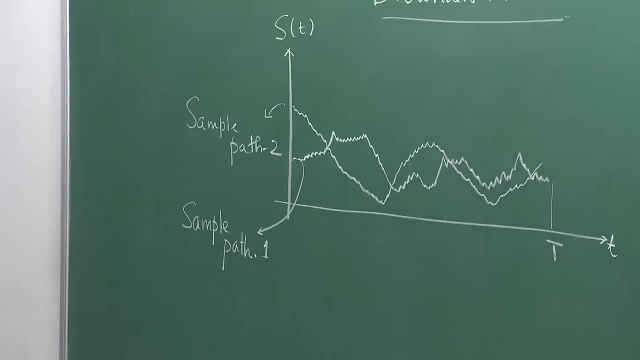 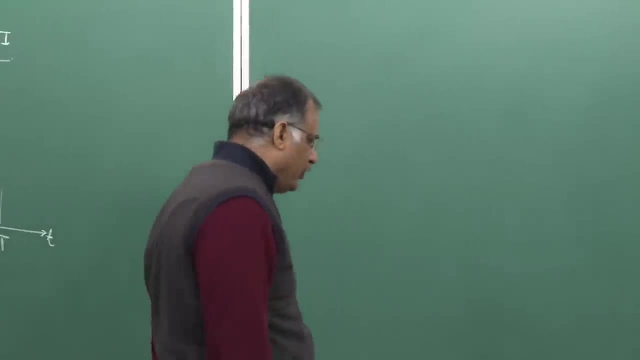 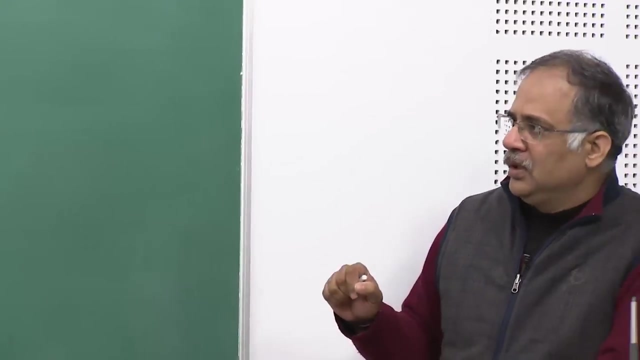 which will help us to model stock prices at the end. So the whole term Brownian motion comes from the name of Robert Brown, who first studied the movement of pollen grains in water and he found that they were having very zigzag, haphazard movements, But it is not so immediately. 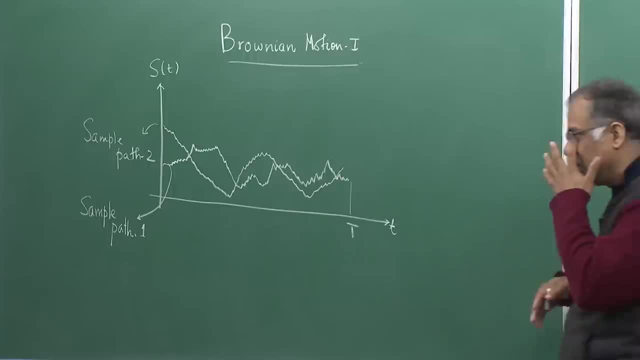 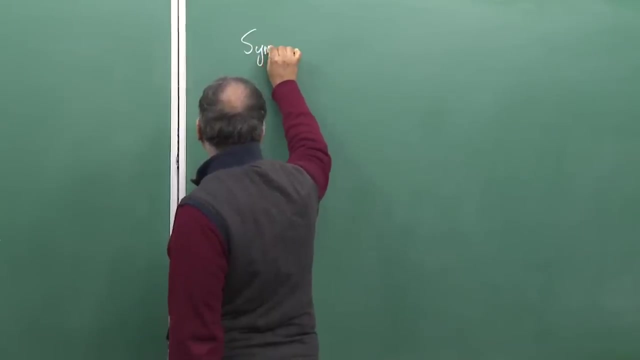 apparent that you can just start writing about this particular stochastic process. We need to have some more idea and build up on some simpler stochastic process. So this will begin. We will begin by introducing what is called symmetric random walks, where there are only two possibilities: You can either go up or down. that is like a coin toss. 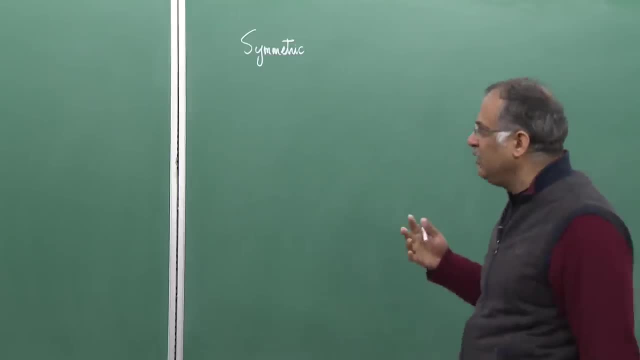 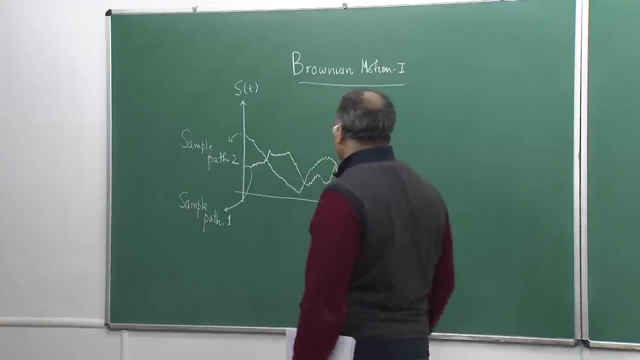 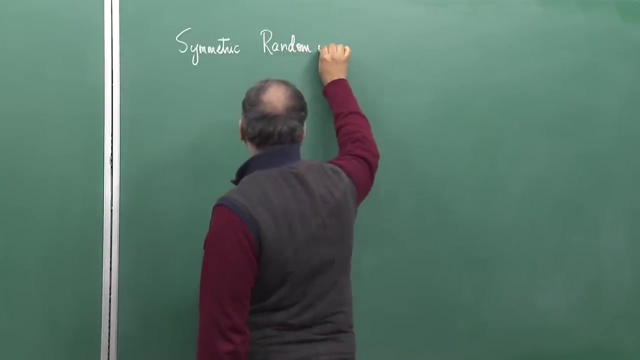 head or tail, and that here I can have infinite such possibilities, infinite such sample paths. Of course there could be infinite possibilities also. Here also we will have infinite possibilities, but generated out of only two possibilities. So symmetric, random walk. So you take a. 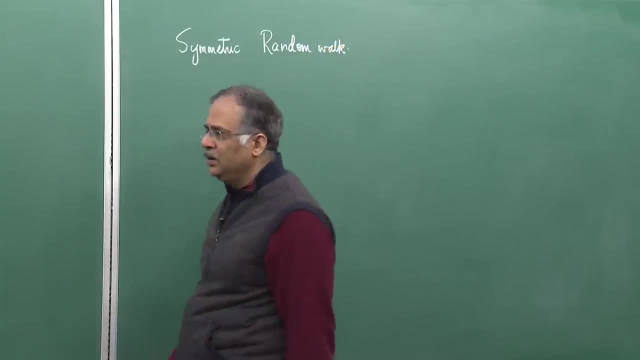 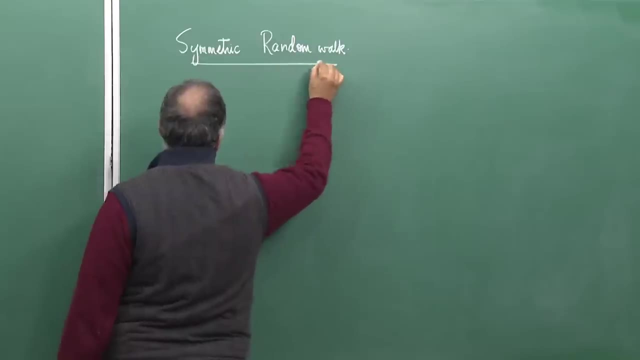 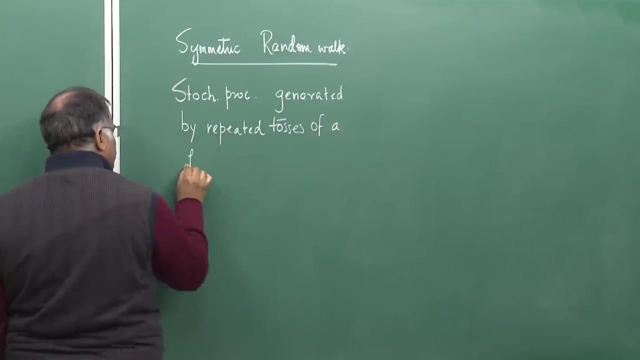 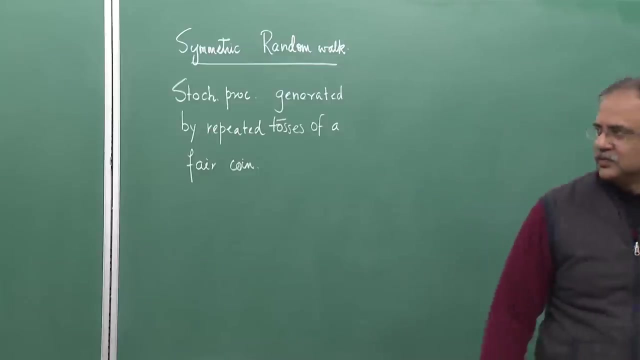 fair coin and then you keep on repeatedly tossing it. So it is a. So this is a stochastic process, which I will write in short from now on as stochastic process generated by repeated tosses of a fair coin, And if you look at it very carefully, what I mean by this. So you start tossing the 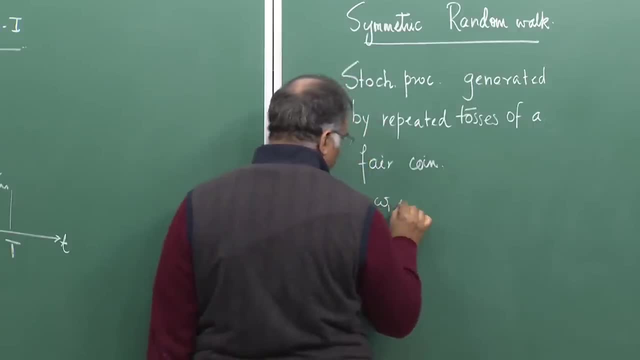 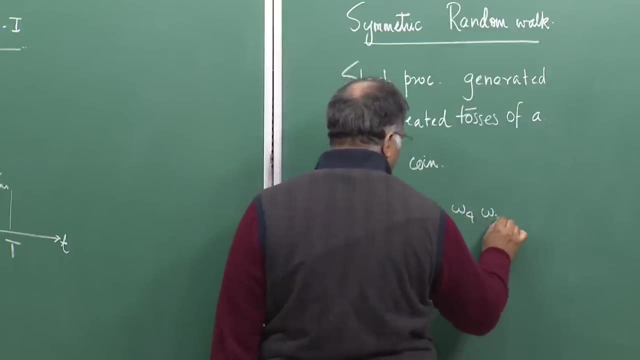 coin. So repeatedly you are tossing omega 1, omega 2.. So omega 1 is either head or tail, Omega 2, omega 3, omega 4, 5 and so on and so forth. Suppose you have here head. head, tail, tail, head, head, tail. So you start tossing the coin, Obviously it will look very similar. It is automatically similar. So the coin: tossesания 한번 by tossing the coin. well, OK, So that means you see this here. So if I just repeat this again, 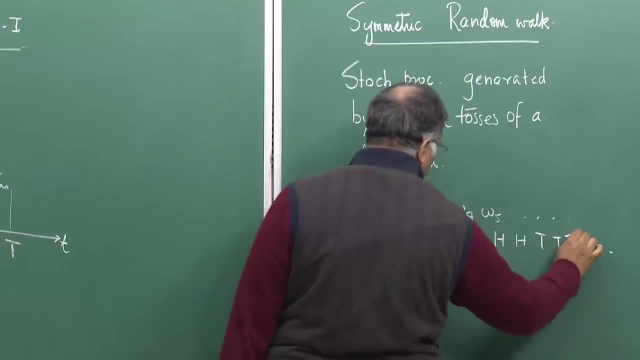 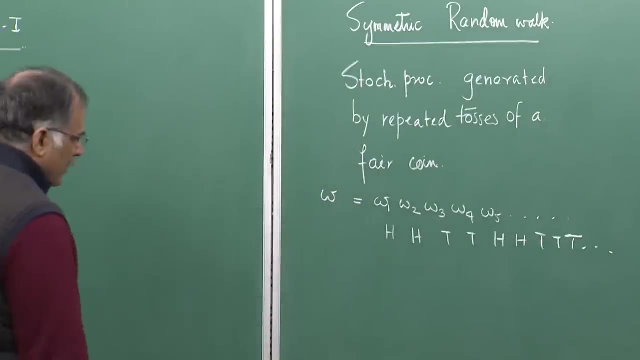 over and over, it remains the same. So you multiply this by stomach crescent市CC, head, tail, tail, tail, and it goes on. So this is one particular scenario that has evolved. You could have another scenario, say omega bar, which is consisting of, say, omega 1 bar. 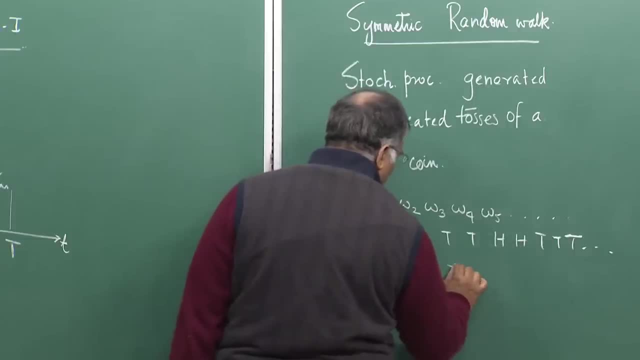 omega 2 bar, omega 3 bar, omega 4 bar, omega 5 bar. It could be something like this: tail, tail, head, head, head, tail, tail, tail, head, head, head, and so on. So these two. 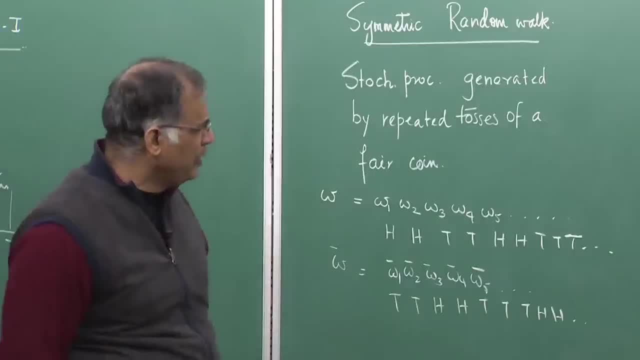 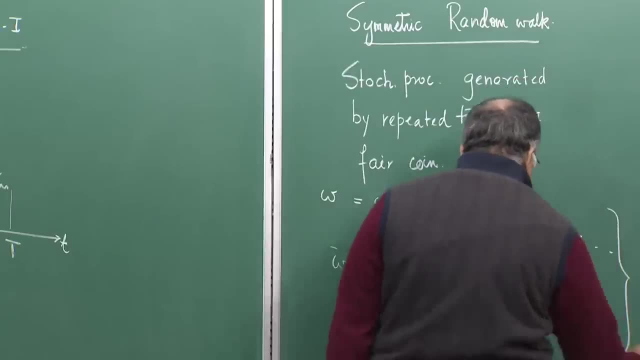 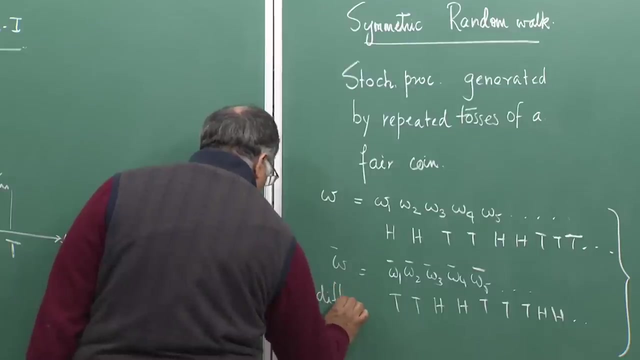 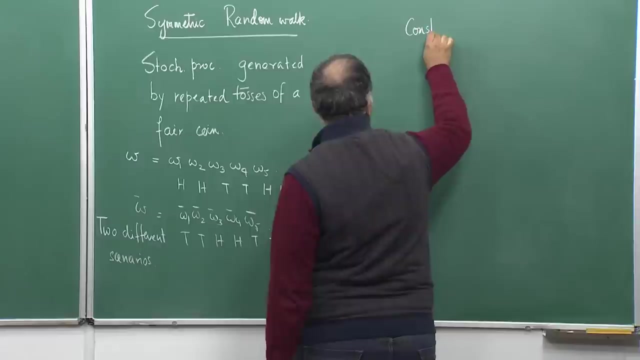 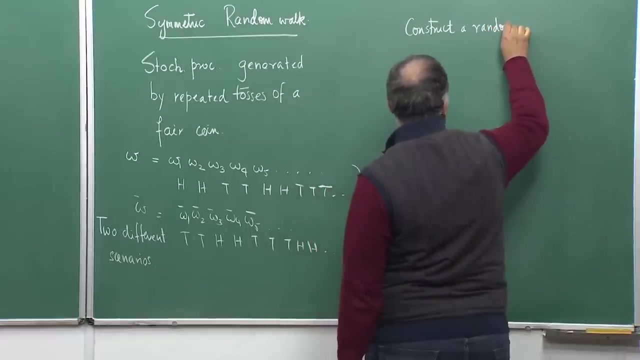 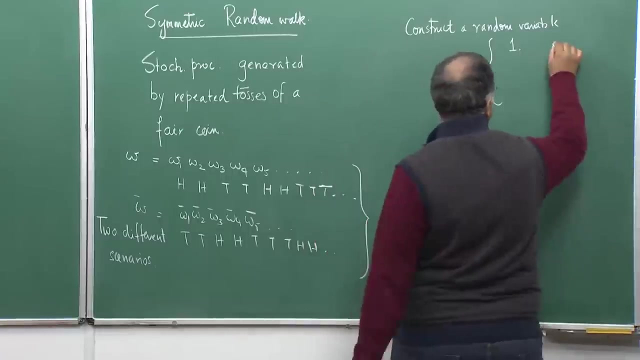 are different scenarios and these two each would generate two different sample paths. So how do we generate this symmetric random work? So these are two different scenarios, two different scenarios. Now construct a random variable: x j. x j is equal to x j, which takes the value 1. if j is equal to, sorry, if omega j is equal to. 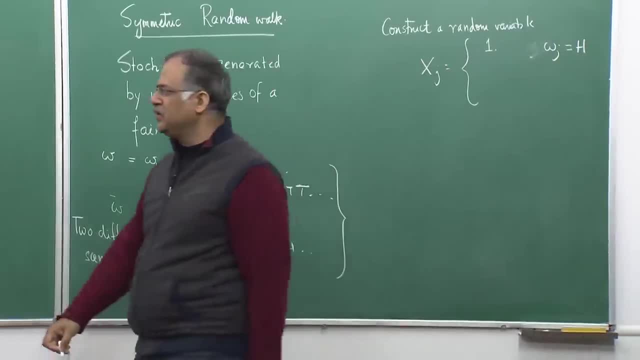 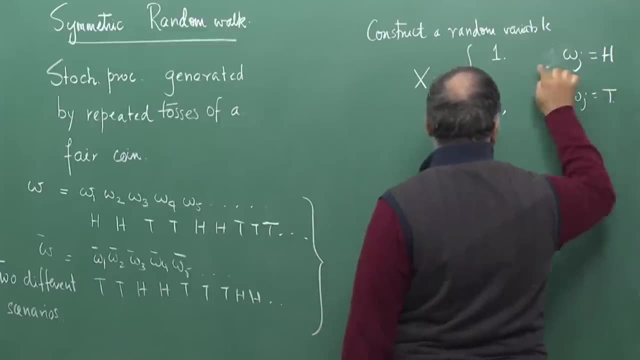 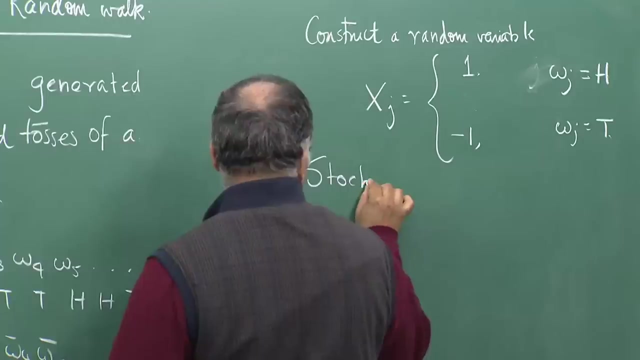 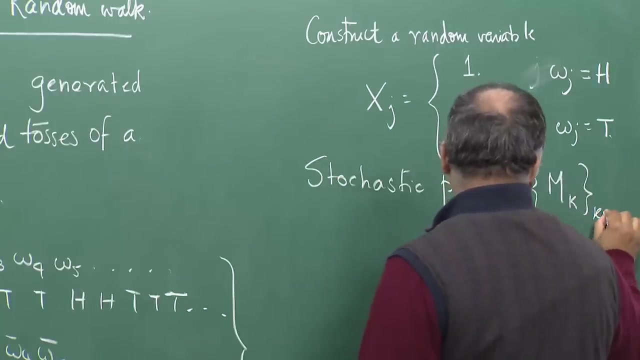 head and takes the value 2.. Sorry, the value minus 1 if omega j is equal to tail, if tail appears, and 1 if head appears. So now you define a stochastic process. So define a new stochastic process: M, k, k equal to 0. 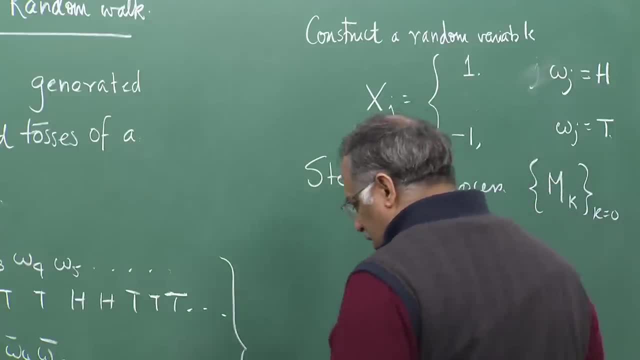 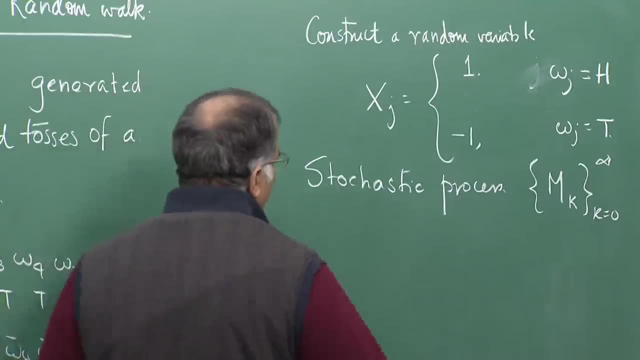 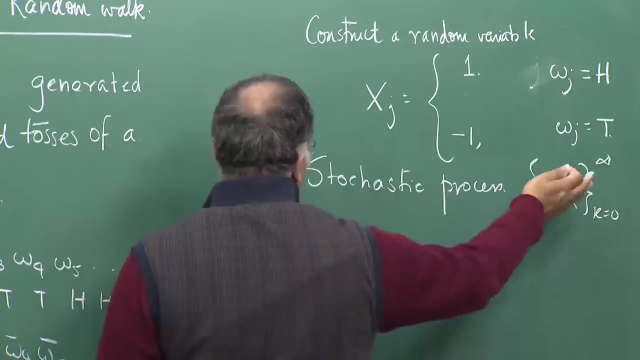 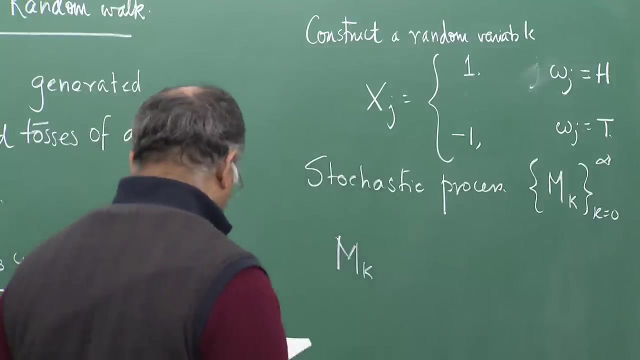 to infinity, or let us- we can in- not bother. we can also fix it up to some time. It could be some time. capital, say k is say 25, something here 25 or 30, whatever. but in general it is alright to take plus infinity, just a sequence where M k is given as follows: Each of these: 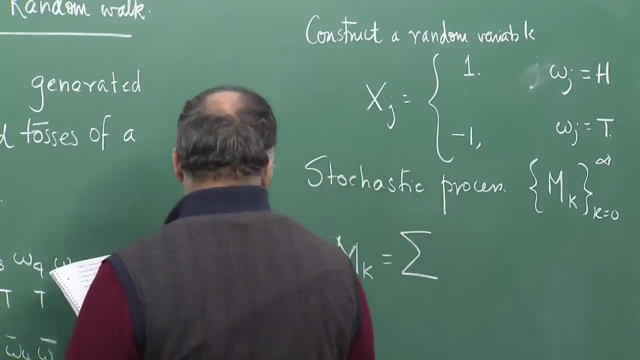 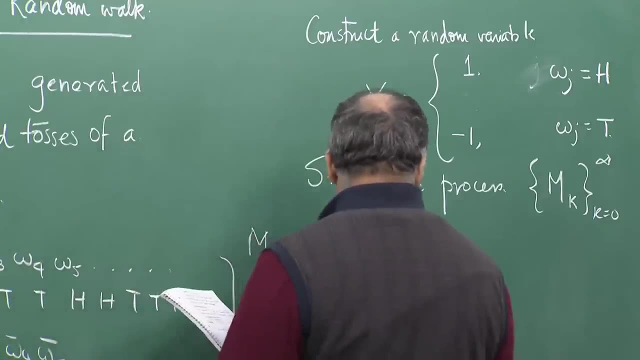 M k's are calculated of 5 to 10 to the power minus 1.. So M k is given as follows: Each of these M k's are calculated of 5 to 10 to the power N, f, by starting from M 0 equal to 0.. M k is equal to j, is a sum from j from 1 to k 3x. 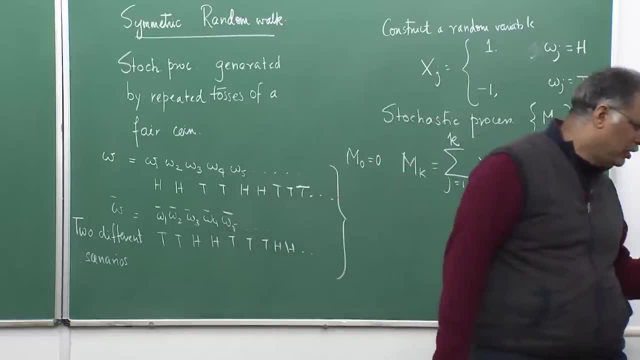 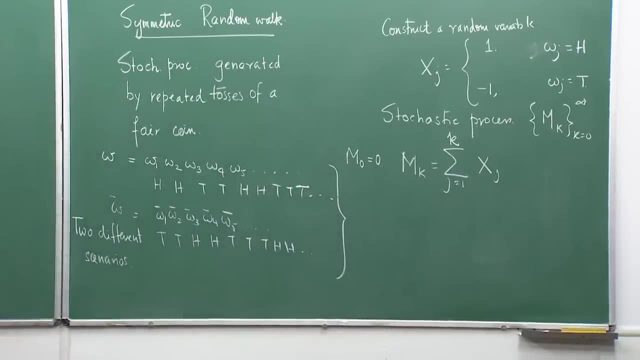 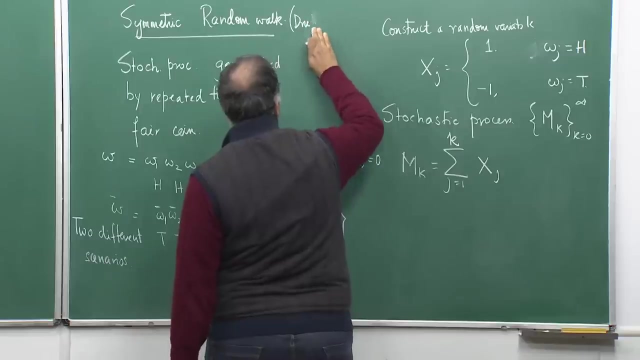 j. Let us see what would happen if one particular scenario like this evolves. Let us see, then, what is the sample path of this. this symmetric random walk is also called as drunkard walk, So somebody has had a good drink and he has become drunk and if you look at, it is his. 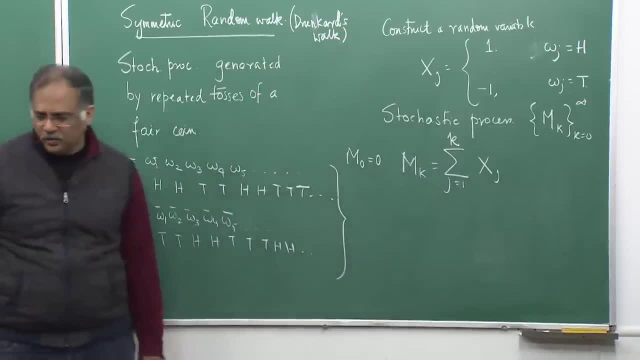 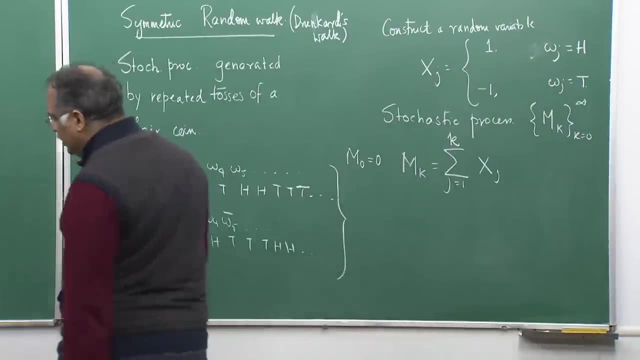 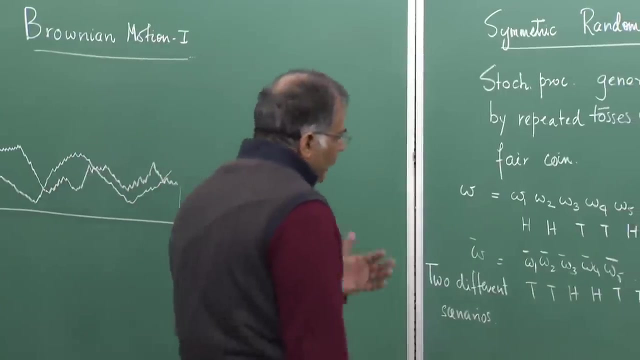 walk. So a drunkard would walk like this: if I am here, So I start from here, then I can just go like this, and he goes like this: just it is just, or like this: you know, I am coming here and then I am going there, something like this, So this sort of thing you will. 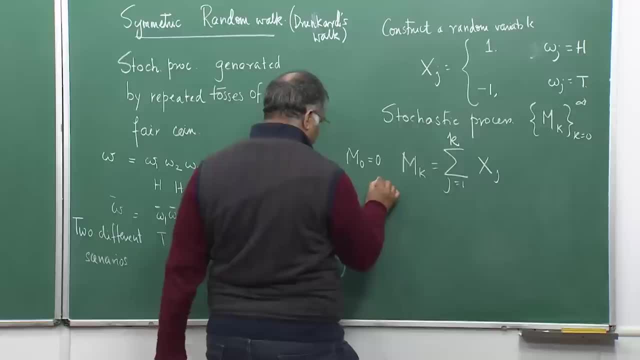 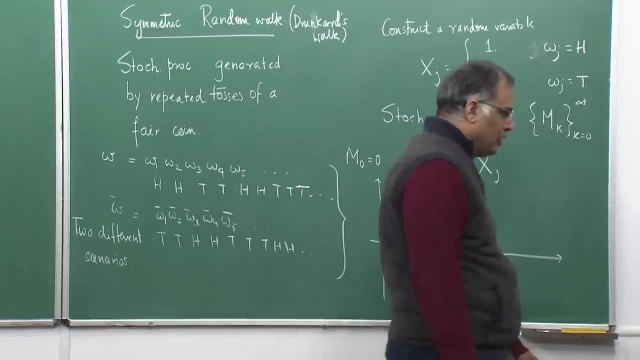 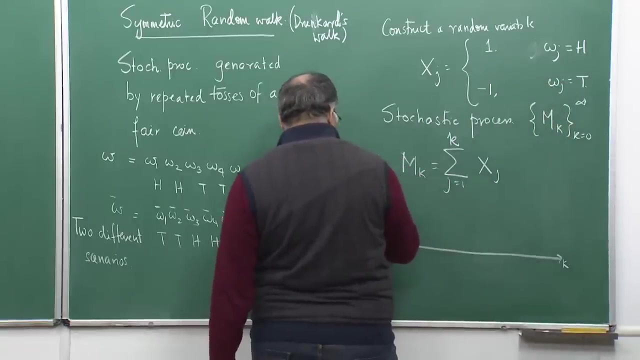 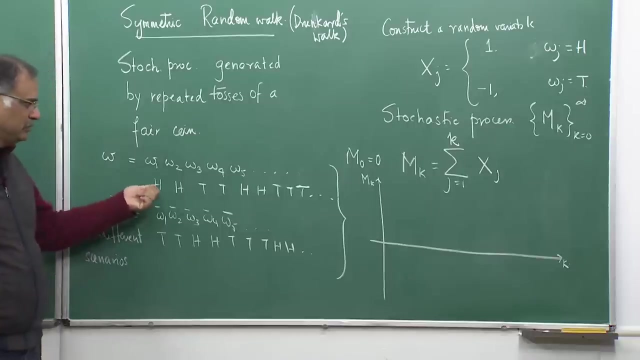 immediately observe as I start, say, checking out with this scenario. So here is my k and here is my m k value. Now, the first one here has turned out to be head. So m 0 is 0. let me write minus 1,, minus 2,, minus 3 and so on. minus 4 here, 1,, 2,, 3,, 4 and so on, And 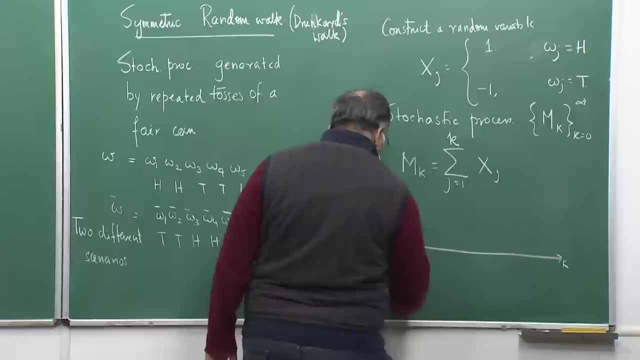 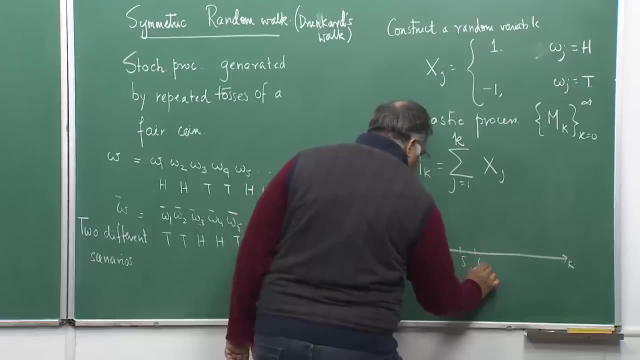 of course that here also you have to have k values, which is 1 or may be not 1,, 2,, 3,, 4,, 5,, 6,, 7,, 8,, 9,, 10 and so on and so forth. So m 0 is 0, this is 0 is 0.. Now you toss. 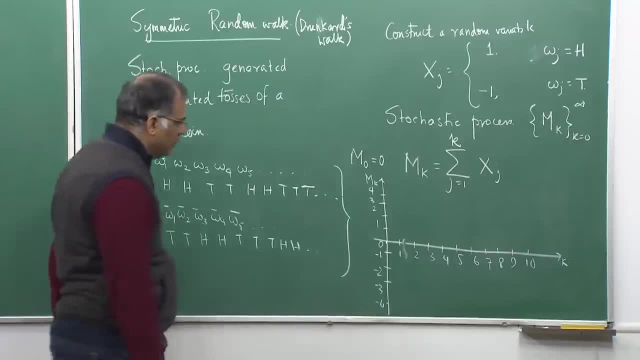 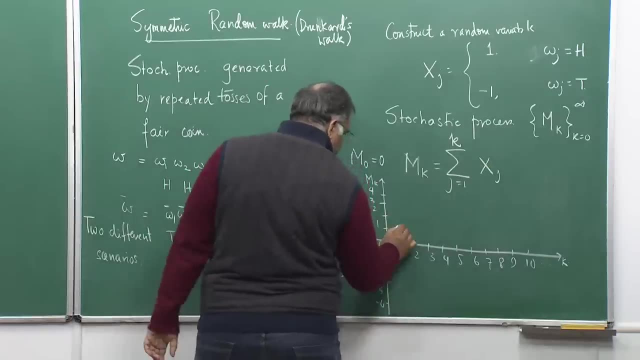 a coin and you have head. omega 1 is head. So you go up by plus 1 because x j will take plus 1 because m 1 is just x 1.. So here is the value of m 1, this is your m 1.. So you, 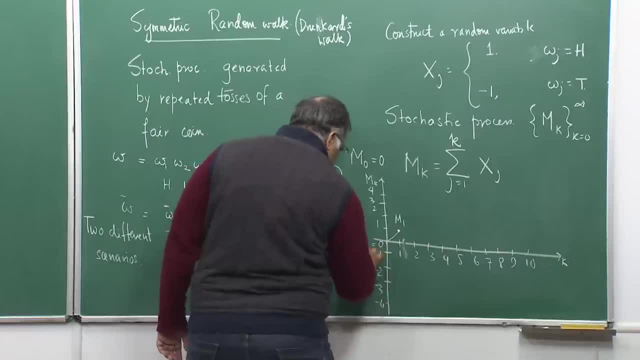 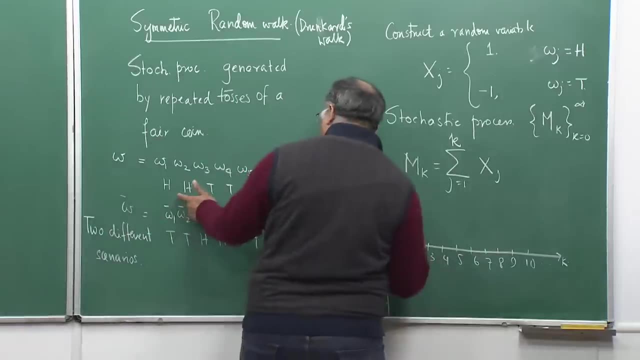 have m 0 and m 1 by line. So 0 is m 0, and then you again at head, So m 2 is again 1.. I am looking at this scenario: m 2 is you go by 1. So it is 1 plus 1 now 2.. So m 2 is. 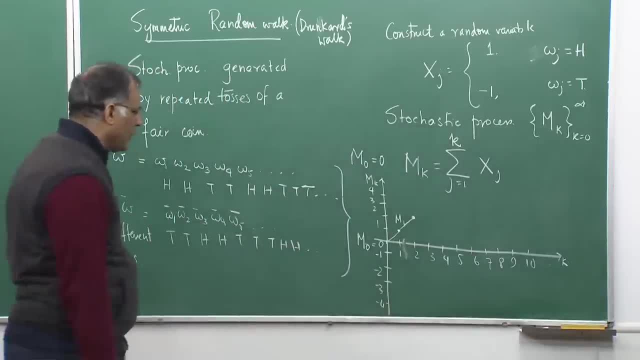 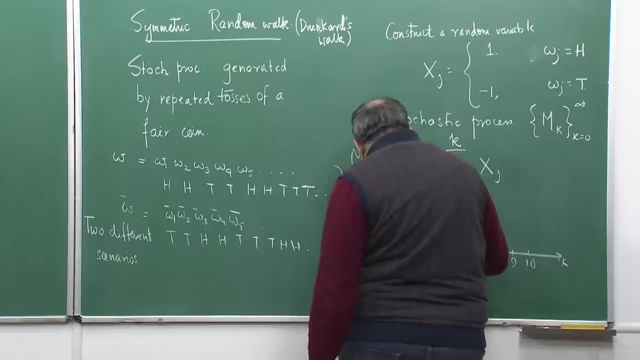 2. So you join again by this line. but m 3 is tail, So you will drop by 1. So it will be minus 1. So you will again drop back to the point 1.. So this is your m 2. So. 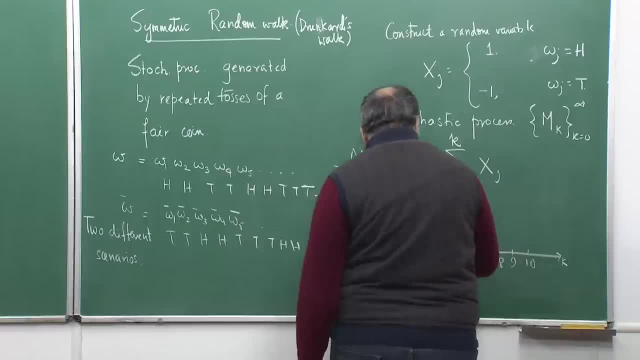 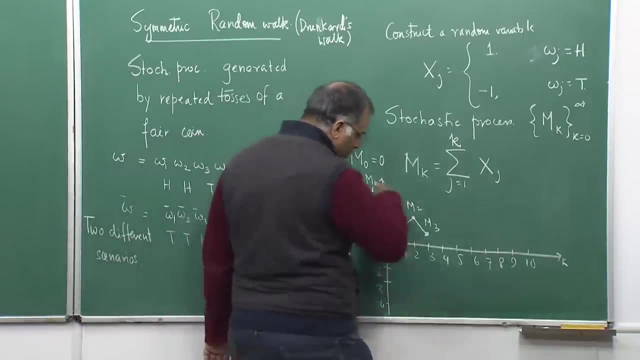 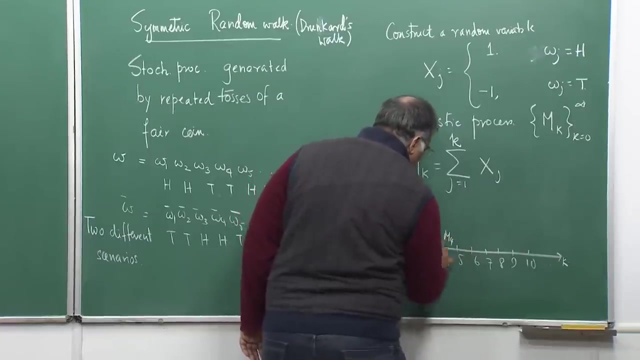 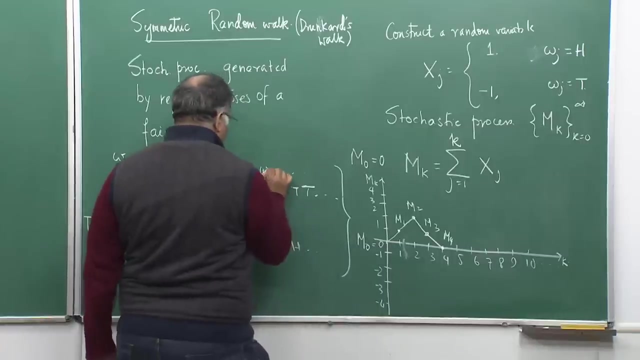 this is your m 3, and then omega 4 is again tail. So drop back to 0 again, you minus 1 subtract, So this is your m 4 is 0.. Again, then you have head for omega 5. say So here. 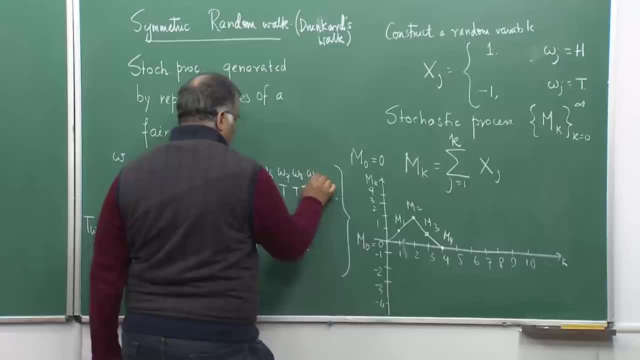 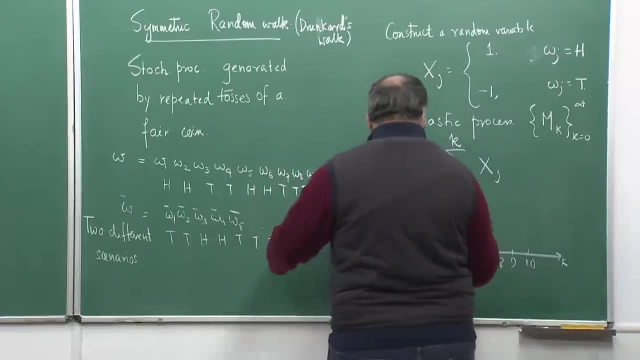 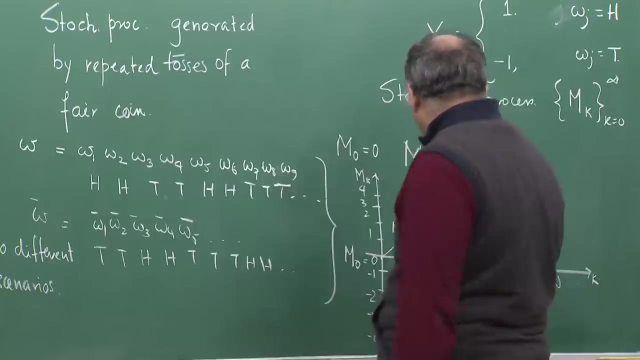 is m 6, omega 7, omega 8, omega 9.. So for m 4, you are tail, you have come to 0 again. Then it goes up again. it goes to plus 1 again. So this is your m 5.. Again, it goes up to. 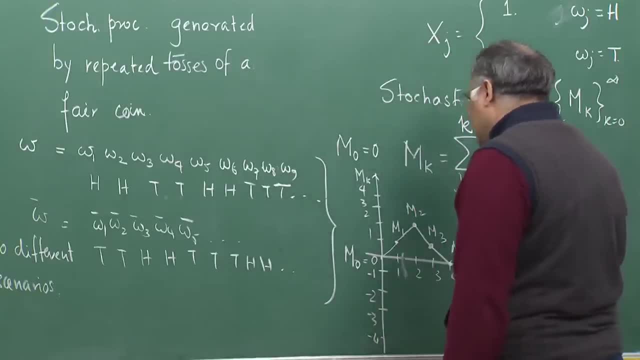 2, m 6, or then you have tail again, So m 7 comes down to plus 1.. Again, you have tail, So M 8 comes down to 0, because you are adding up everything at every step you are going. 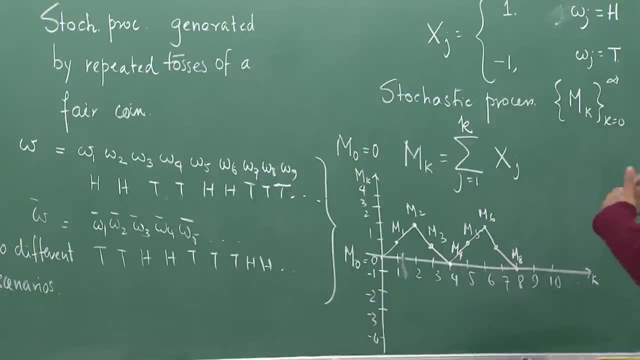 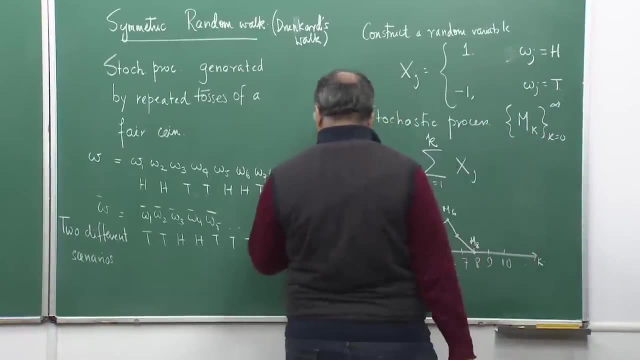 up or down. So you add up in this fashion and you move like this. So M 8 I have here, omega hat is again, omega 9 is tail. So again I have to go down. So I go down by. so from: 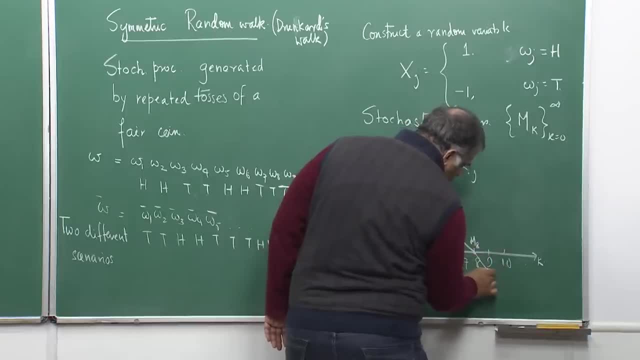 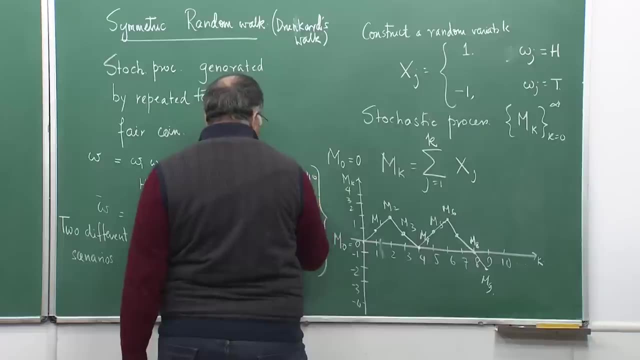 0, I will have to go down by 1.. So I will come to minus 1.. So this will be your M 9, and if suppose M 10, omega 10, is head, then it will again go up to 0 at the 10th place. 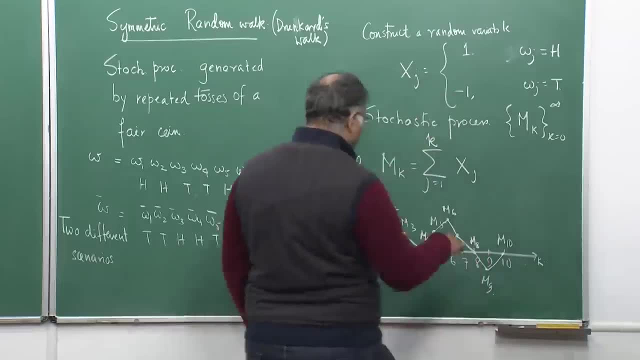 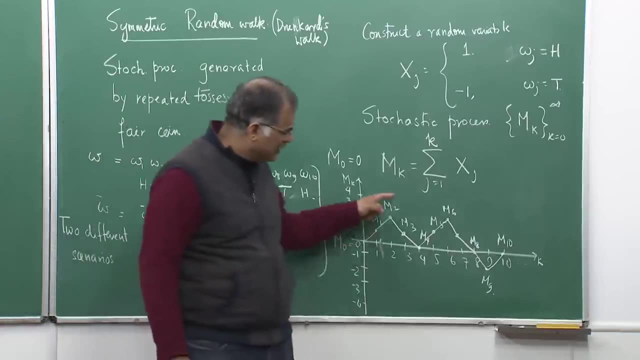 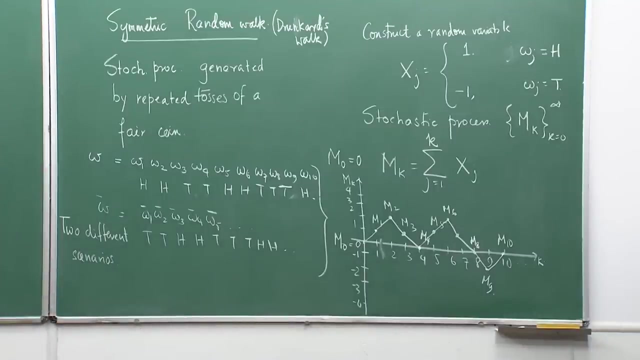 because it will again add 1.. So it will become your M 10. So what? you see that the symmetric random walk is providing me some zigzag looking curve. So Which might tempt you to think that possibly these two have some relationships. They are. 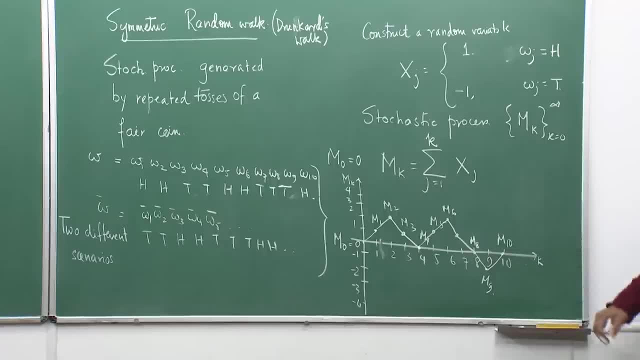 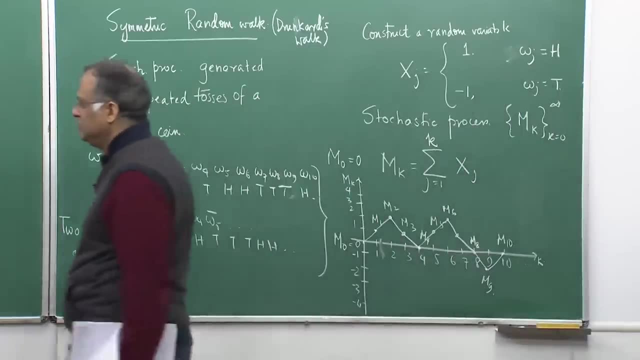 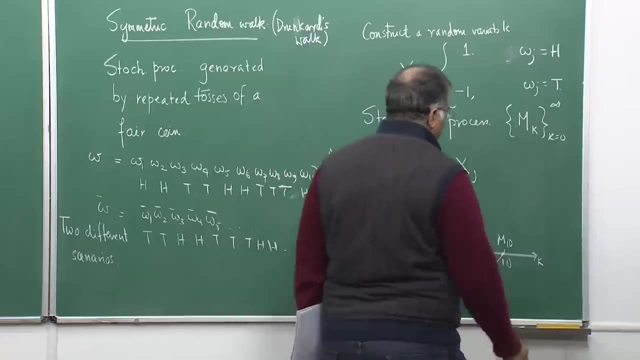 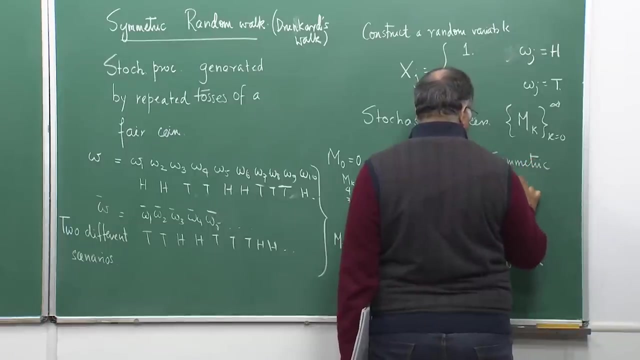 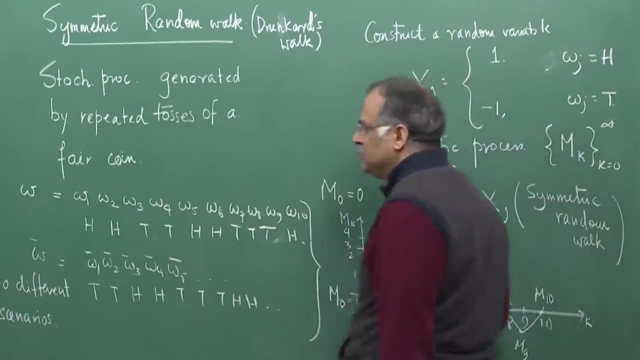 they do have some relationships and we will talk about that slightly down the talk. But let me tell you some more properties of this symmetric random walk M k. So here is my stochastic process and this stochastic process is called the symmetric random walk. Of course we are not mentioning what underline. we are always taking some probability space. 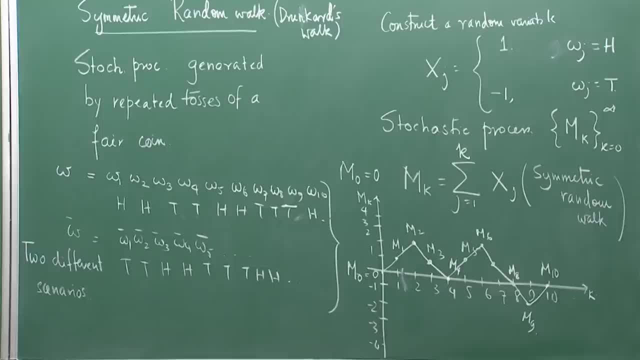 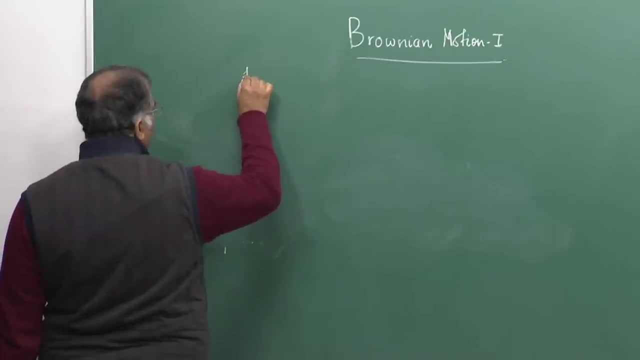 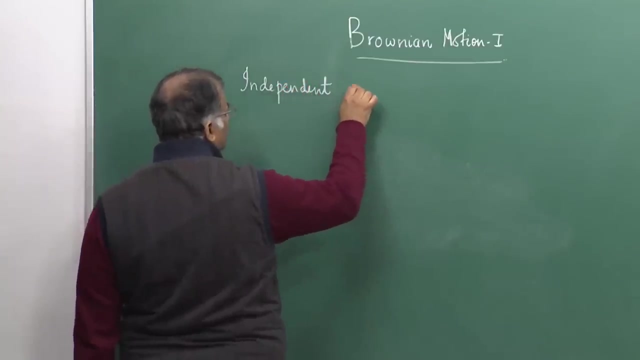 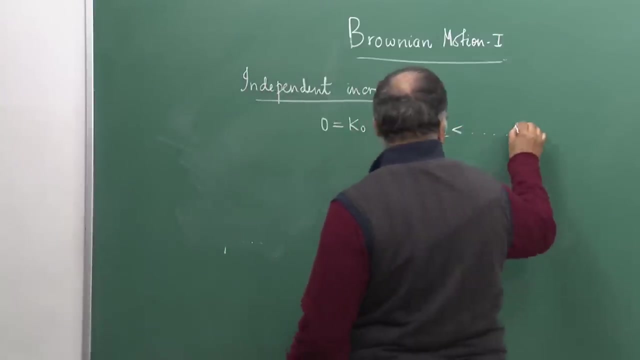 and all of those things. So now we will these random, this particular random process or stochastic process, as independent increments. What do I mean by the fact that they have independent increments? What I mean is the following: So if you have to take certain numbers sometime, say some k m, then you have 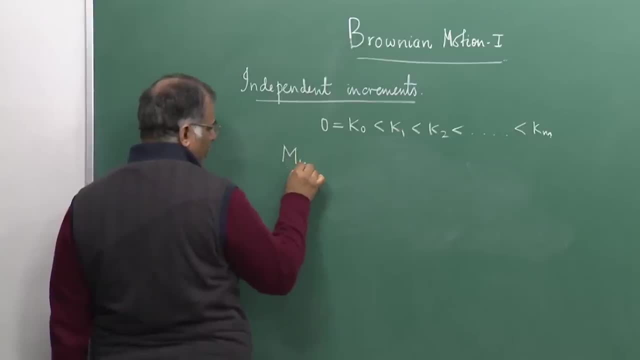 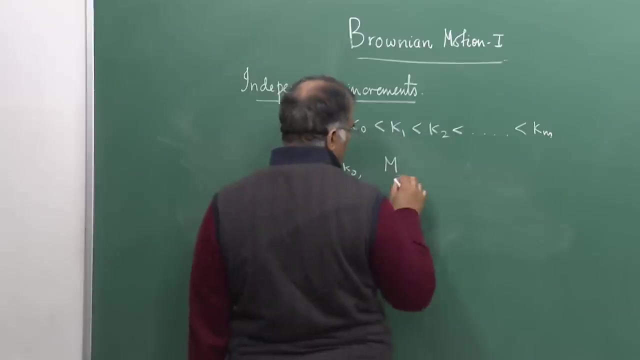 the following: You have m k 1, that is, once you consider non-overlapping intervals. then this difference is independent, because they depend on independent coin tosses. because coin tosses are independent, The coin toss at the second level really does, not the second. 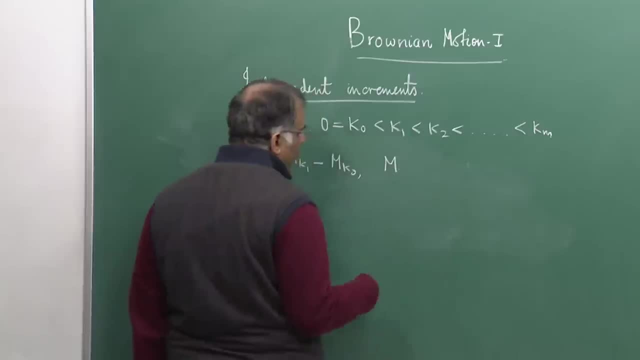 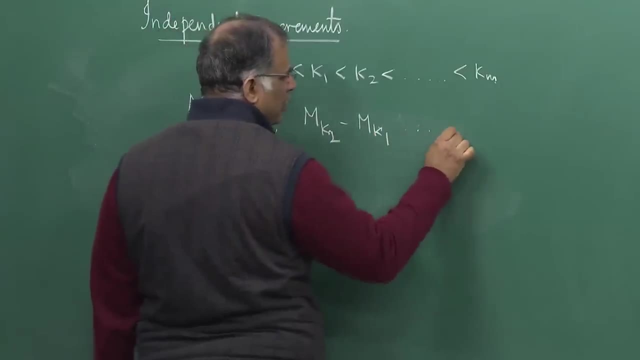 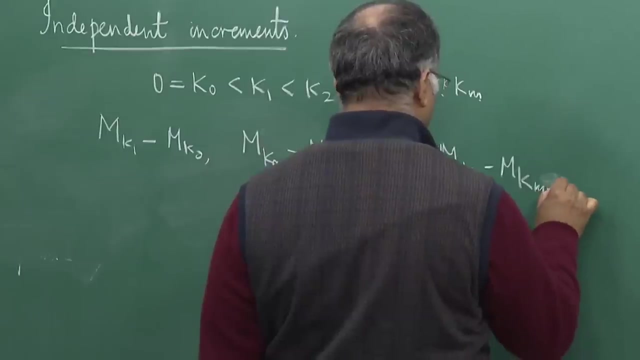 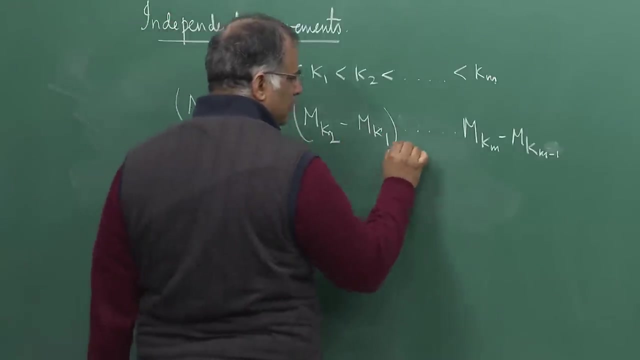 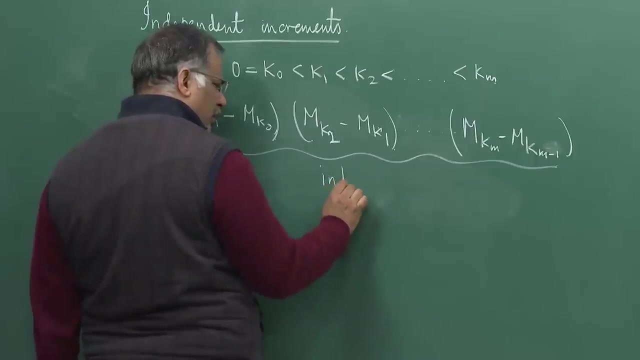 outcome does not really depend on the first outcome when you do a repeated coin toss- Sorry, k 2 minus k 1, m k m minus m k m minus 1.. So these random variables are independent, All of these random variables. these form a set of independent random variables. So 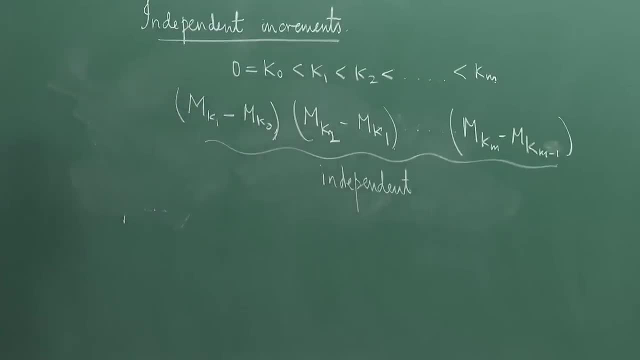 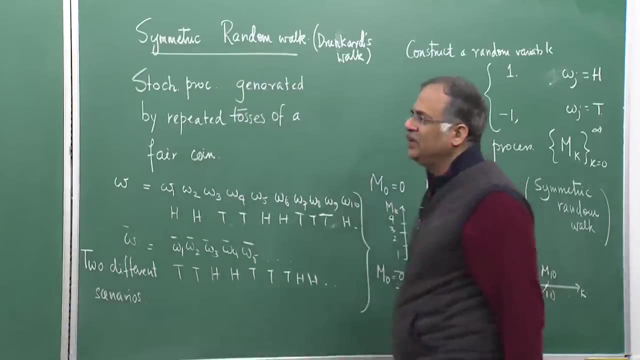 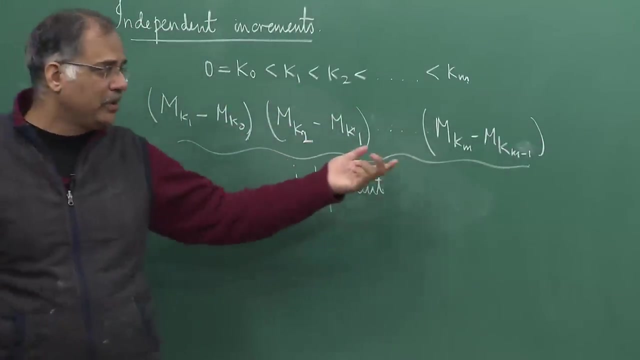 that is, once this happens. This is when we say that it has independent increments, and this actually has independent increments. These are independent because their difference, which really does not depend on the coin tosses here, does not depend on the coin tosses here and here. So you have. 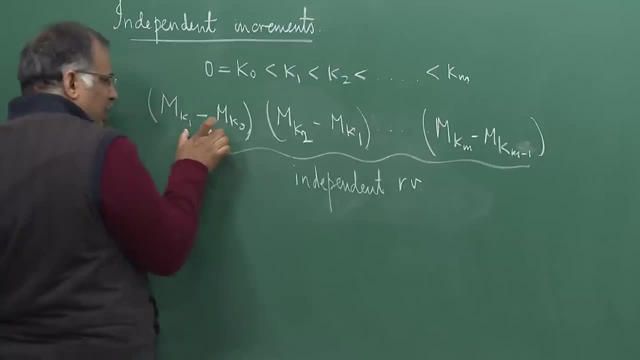 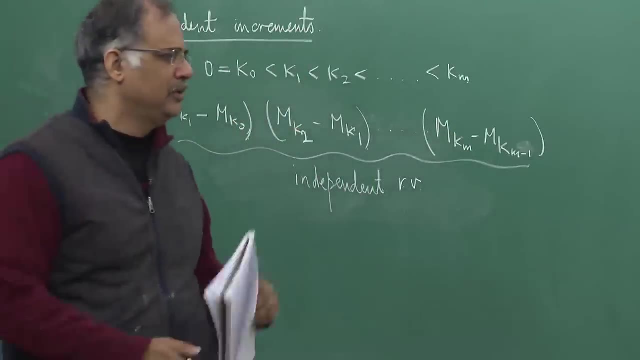 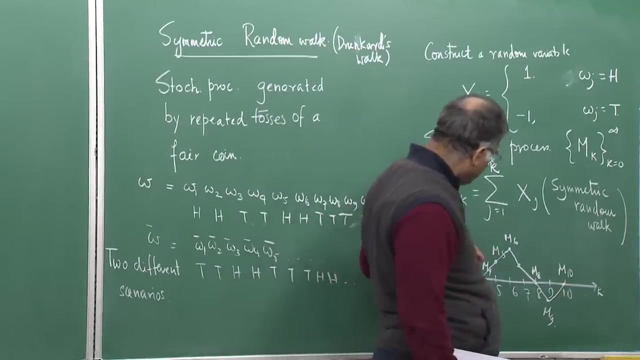 independent increments. So this change that you see here does not depend on the change that you see in this interval or the change that you see in this interval. So you can still observe that it is like a drunkard walk. So drunkard walks like this: 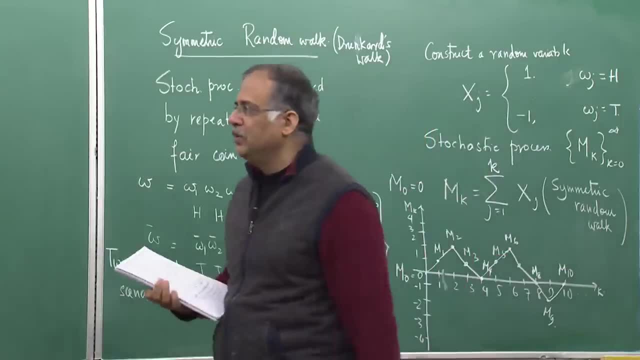 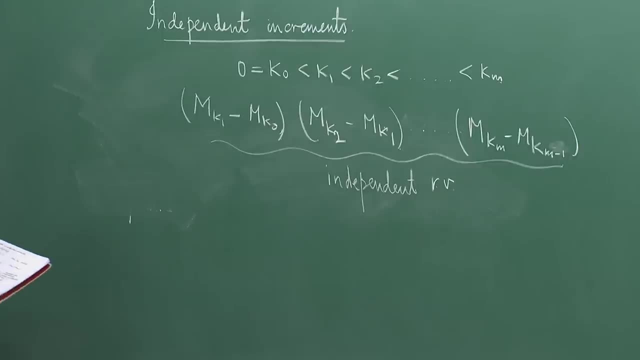 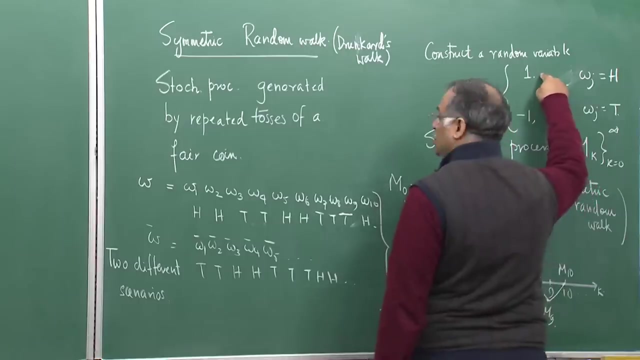 goes down, goes up. In George Gamow's famous book 1,, 2,, 3, infinity- this has been described in a very, very nice way. How do you see here my success? probability: This occurs with probability half and this also occurs with probability half. So if you observe that exponential 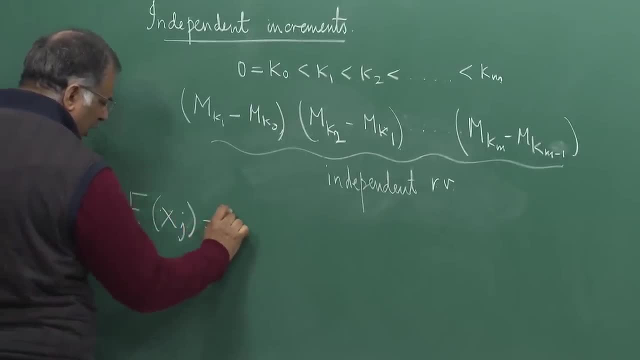 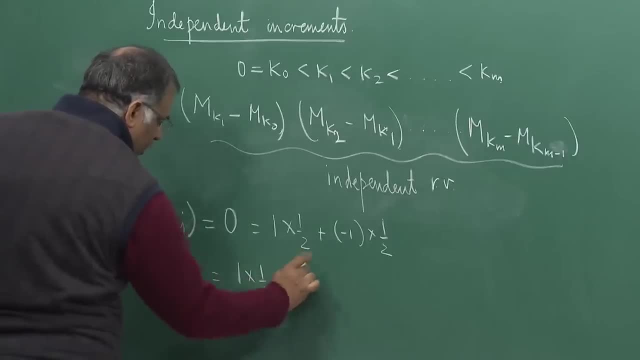 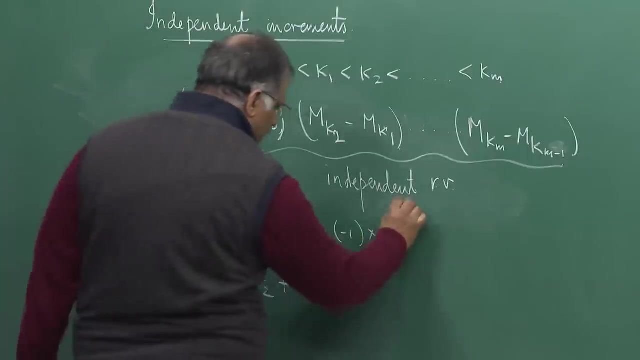 is 1 into half plus minus 1 whole square minus 1 minus 0 whole square plus 1 into half, which is 1.. Once you have this information- this is true for all j- it is immediate that you have to assume that. 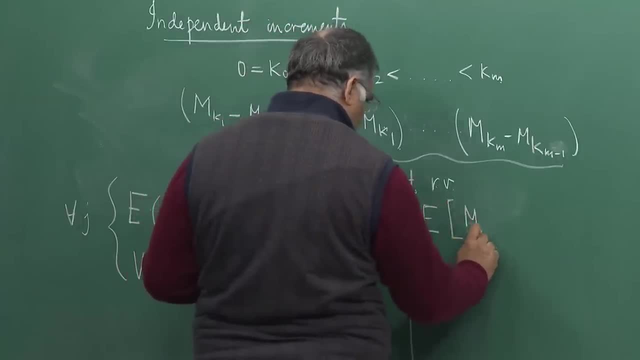 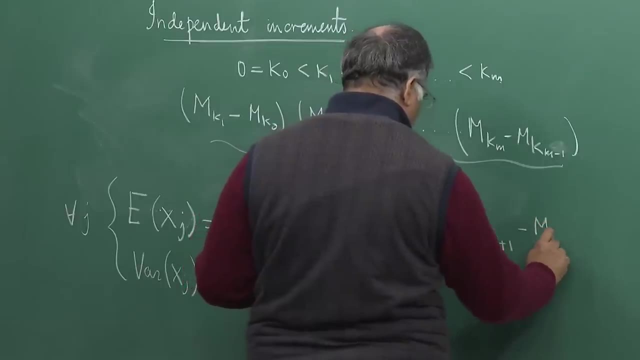 In this case, the variance of x- j is 1 plus minus 1 cube and the different j's that are executed, the variance of x- j is 1 plus 1 cube, So it is 1 plus 1 cube, In order. 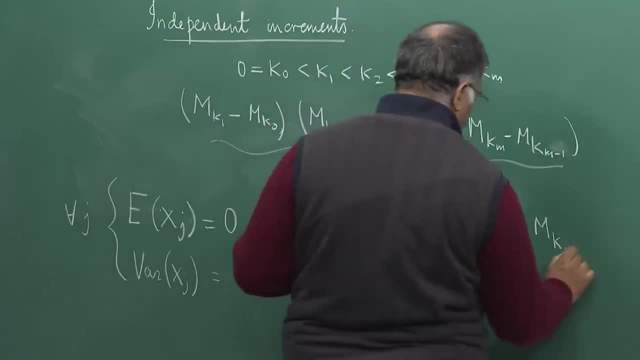 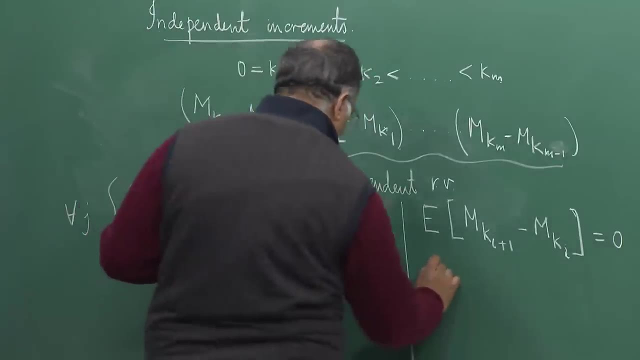 to be sure that the variance is 0, we have to have the verification of the j's. So what is the variation of x? j? The variation of x? j is 2 into half plus 1 into half. It is 1 into half and the various j's are leaving. So this is the variance of x j: 1 minus. j 2 is 1.. So it is 1 into half plus 3 j 1 minus 1 cube. What does it mean? J j 1 minus 1 is 1 into half plus 1 cube. So this is the variance of x j minus 1 cube. So you can see that when you are. 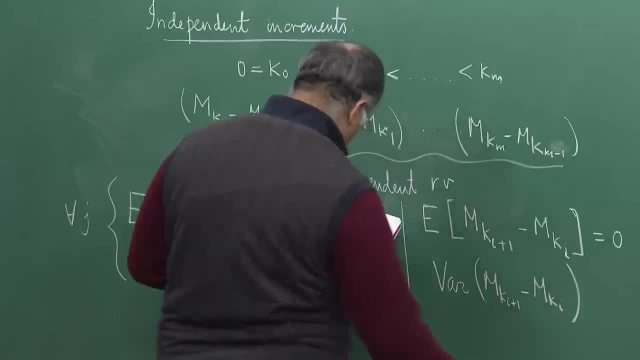 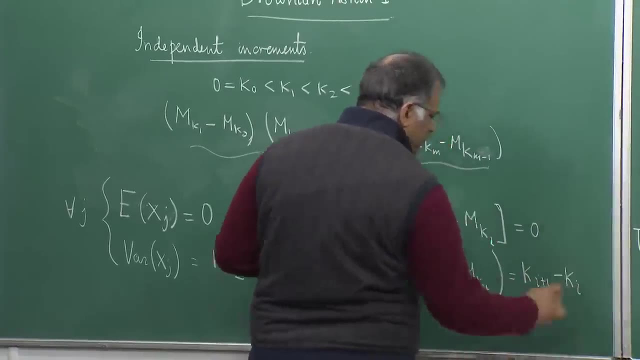 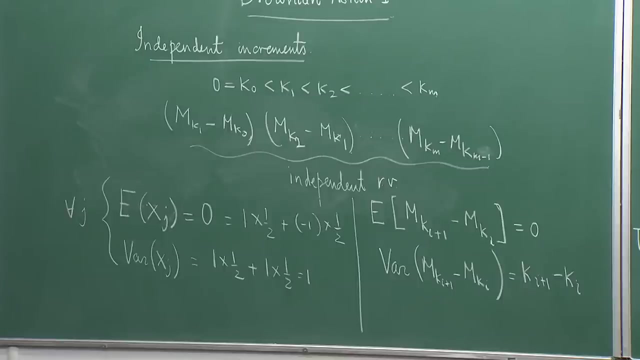 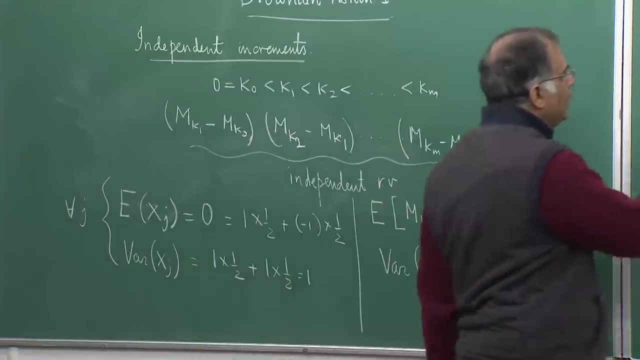 1 minus m of k i is equal to. I leave it to you to calculate this stuff. Our second property about this random walk is to show that this is also a martingale. You see, martingale thing comes up. So symmetric random walk is a discrete martingale. 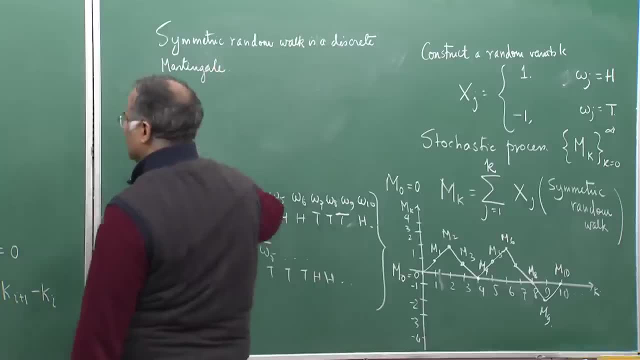 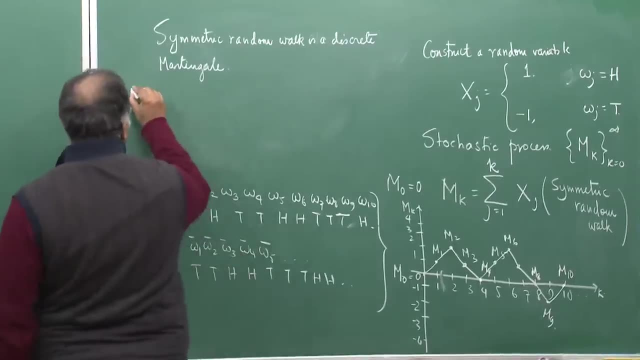 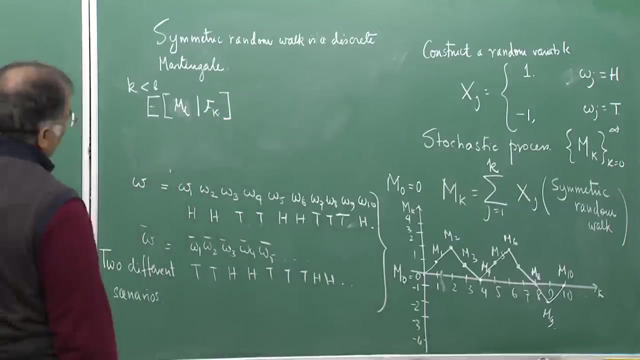 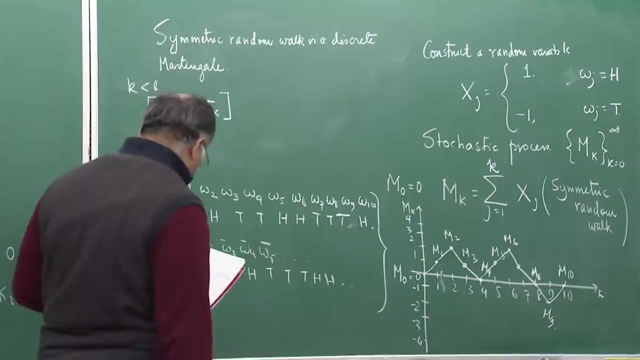 So you can easily prove that it is a martingale. So you take any k strictly less than l and look at the expectation of m l conditioned on the filtration, the sigma algebra f k, which is a part of the filtration. So you can write this as m l minus m k plus m k. So this can be summed up just like expectation. 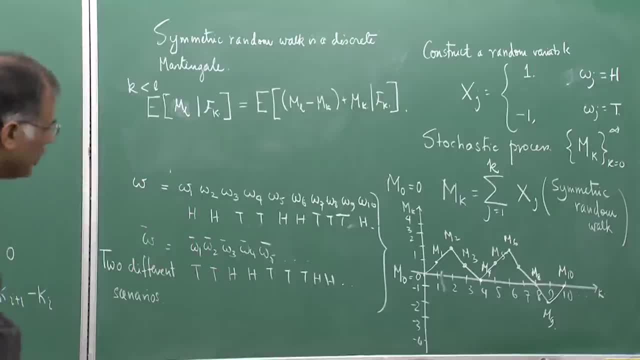 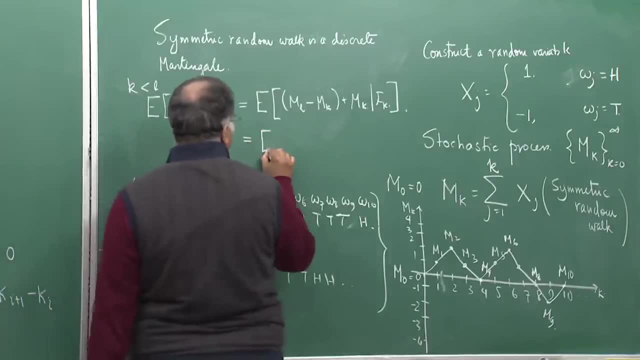 can be summed. So this random expectation, this random variable can be decomposed into two parts which you can actually prove, which will be a part of your exercise. but we are just using this fact here, So maybe I should drop the board a bit. 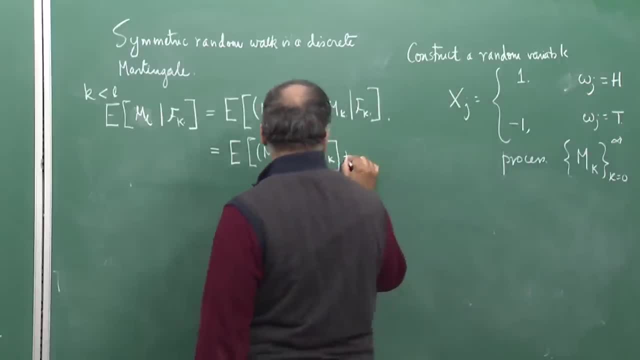 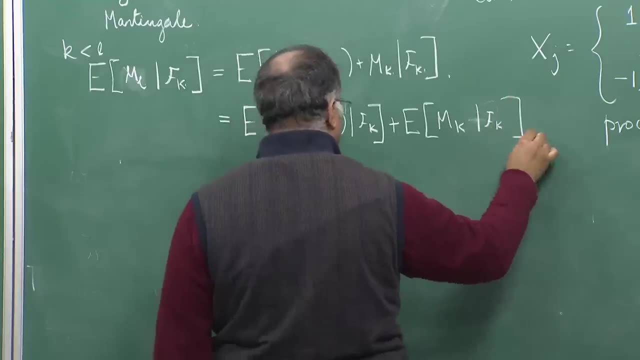 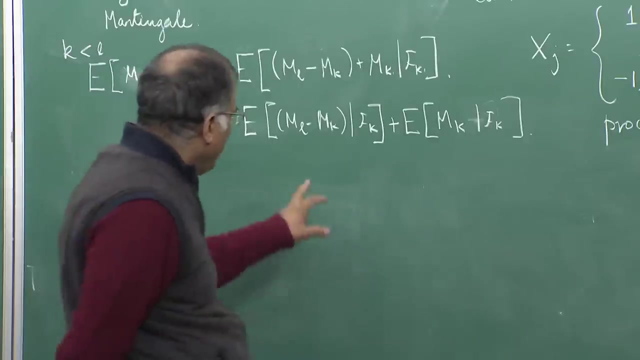 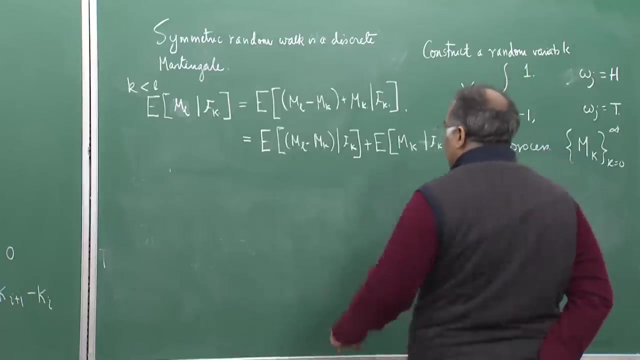 So this is what I am saying. Now let us look at the first part. Since l is strictly bigger than k, this increment, m l minus m k, is independent of f k. f k does not have a information of anything, which is: 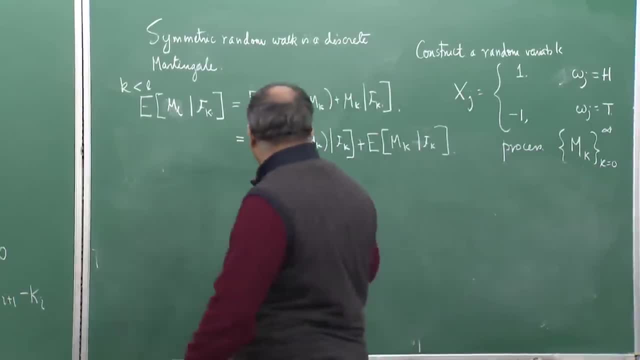 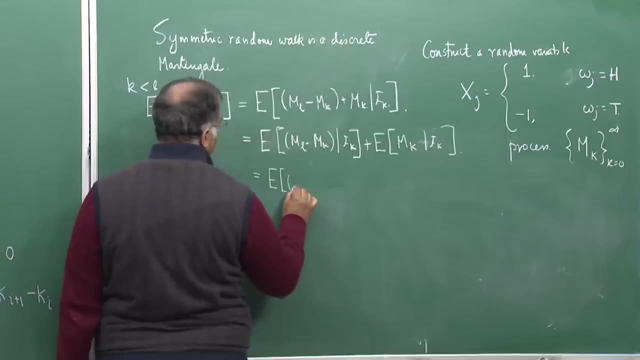 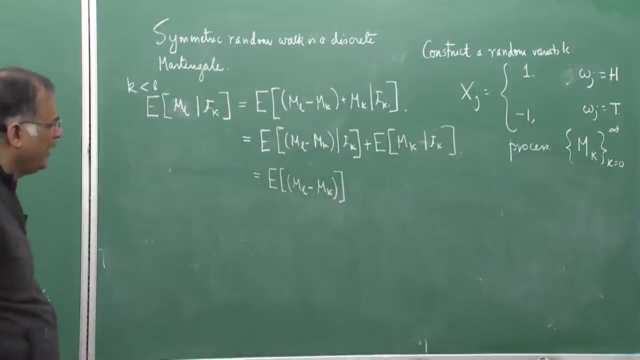 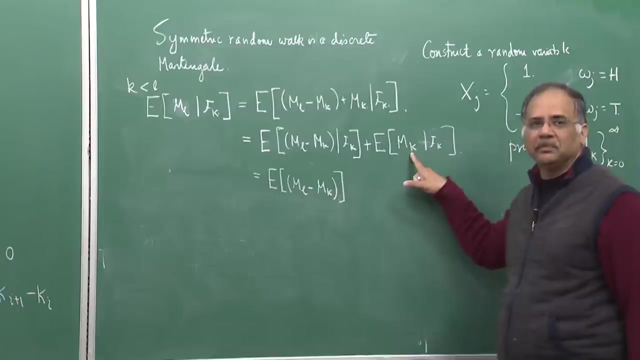 beyond the time k. So here, by our one of our rules, we can say that this is the time or one of our rules for conditional expectation. This is nothing but m l minus m k. Here, at time k, everything about m? k is known. So f k contains all information about m k. So 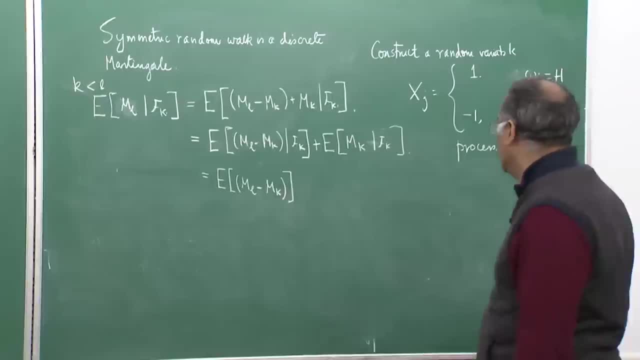 we have we. the first law was taking out what is known. I can write this m k as m k dot 1.. Where 1 is the constant random variable 1.. So I am getting this as m k. This is a. 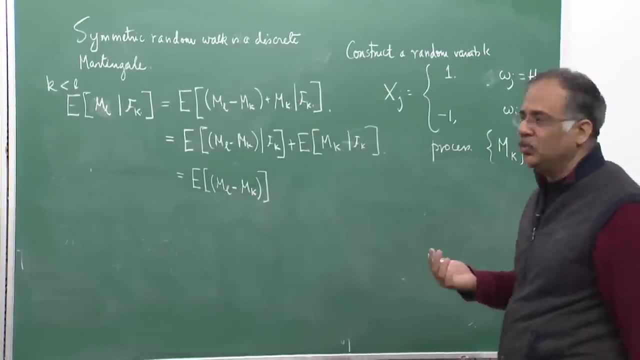 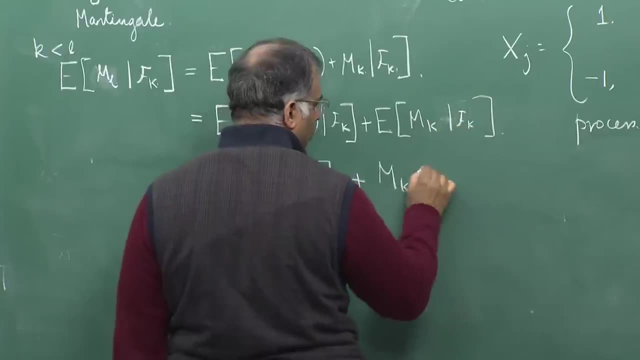 variable 1.. So, whatever be the scenario, it will just give you the value 1.. So I can write this as m k. So I write this as m k dot 1.. So it will. So I can take out what. 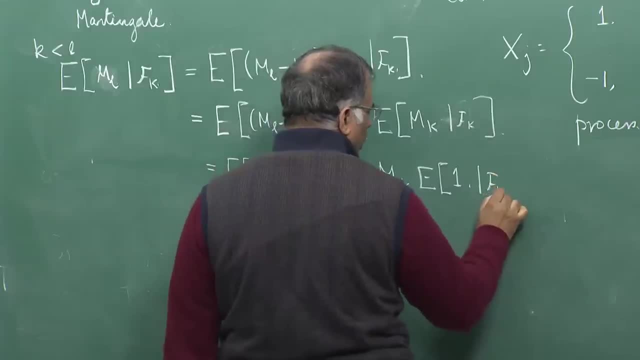 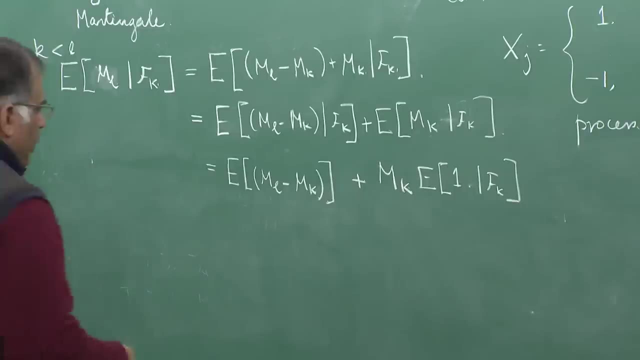 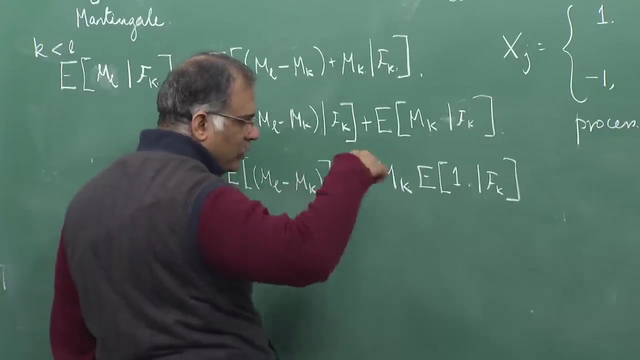 is known 1 dot, f k. Of course, 1 is a constant, random variable. It does not really depend on, is independent of f? k. So it will be E of 1, which is a constant, which will be just 1.. So everything will be 1.. So the sum of the probability will sum up to 1.. So the 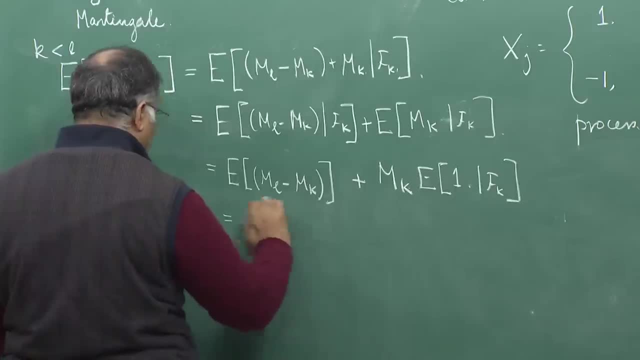 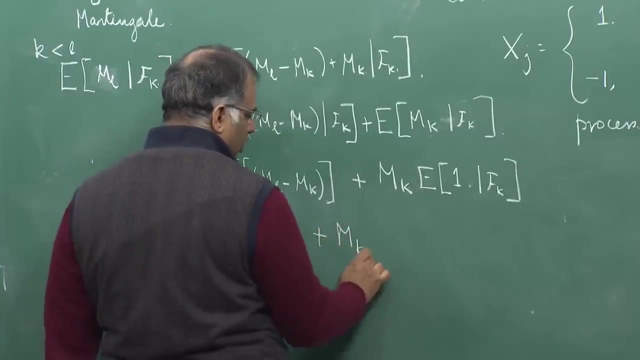 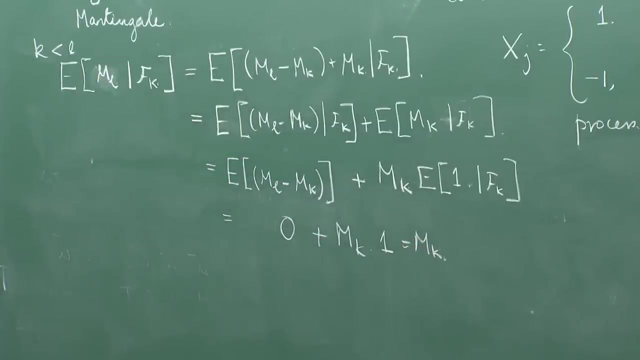 expectation will be just the number. So this again is 0, which we already know, plus m k, into 1, which is m k. So this shows that m l is a symmetric random walk. This thing forms a discrete martingale. 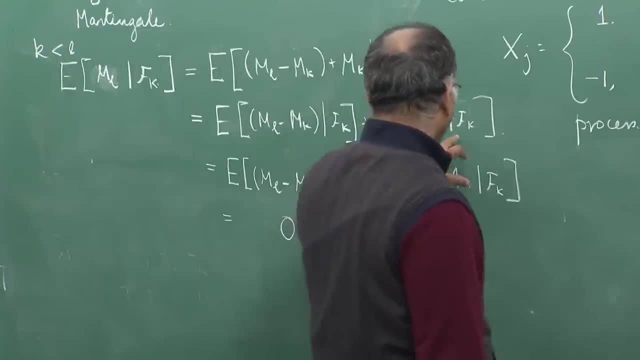 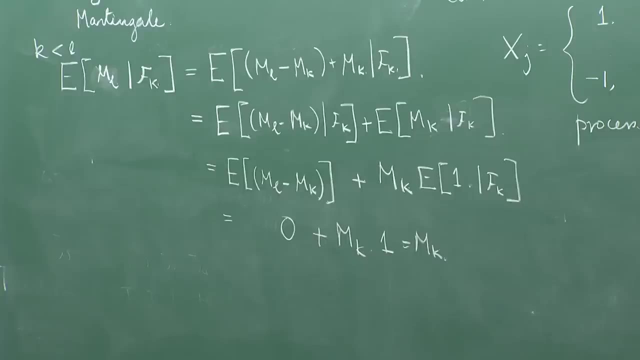 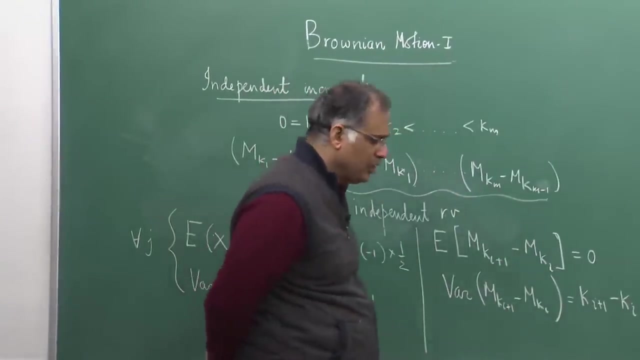 Of course f, k is m. k has to be adapted to this filtration. That is the basic definition of martingale. There is another notion which crops up in the study of these sort of processes. It is called the quadratic variation. So you essentially look at path by path. You 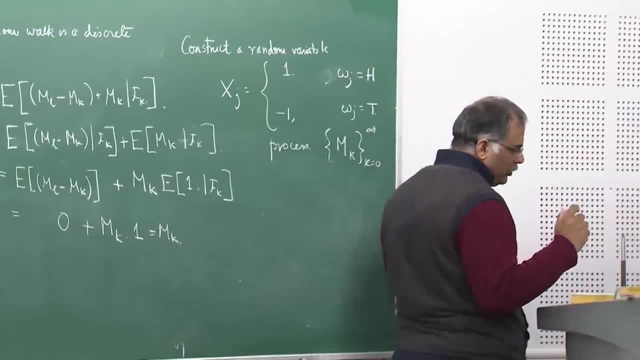 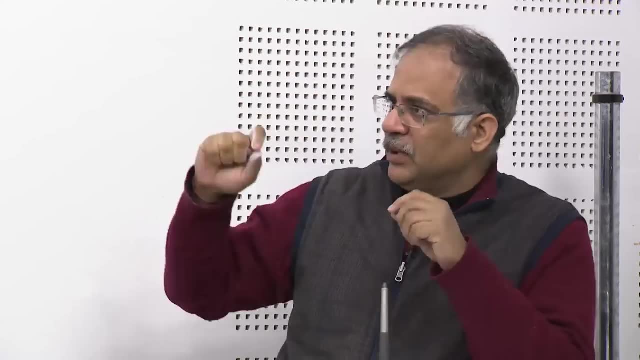 look at how much the random variable values are varying between one end of the path to other end of the path, That is, between k 1's and k 2's. say How much it is varying. It is varying, but do not take just the sum of those variations. They may just be 0. So 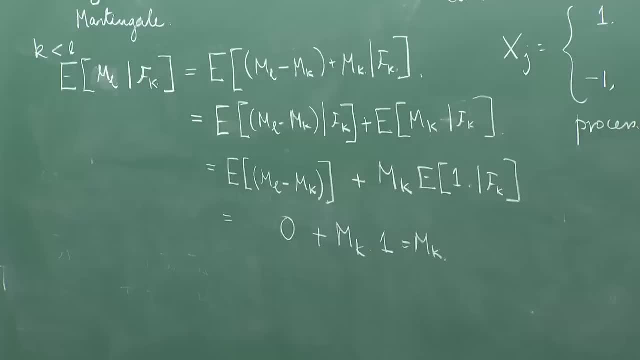 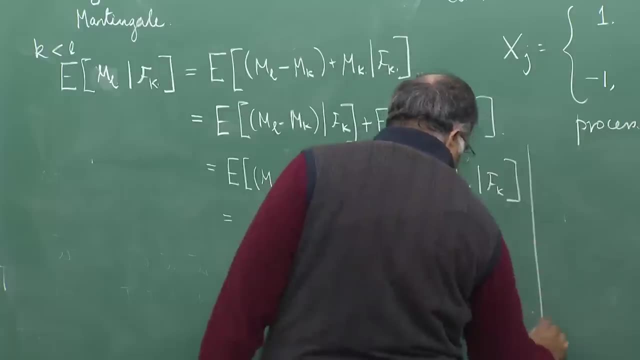 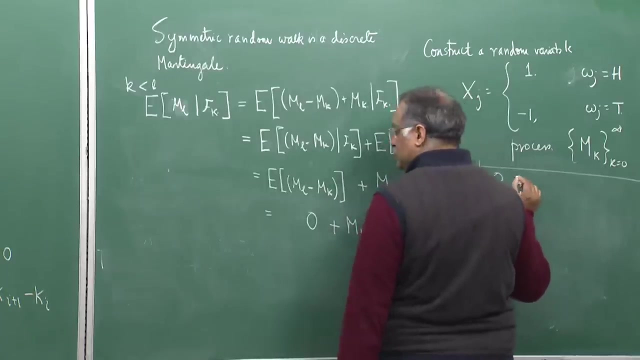 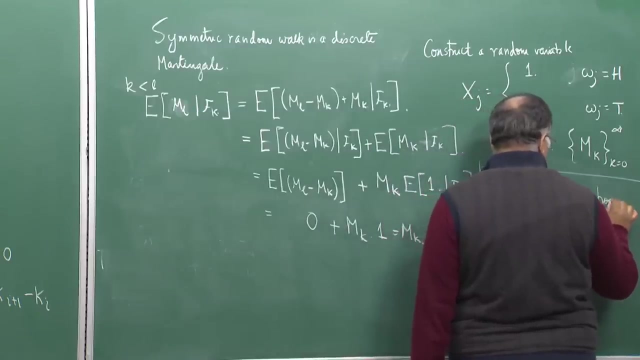 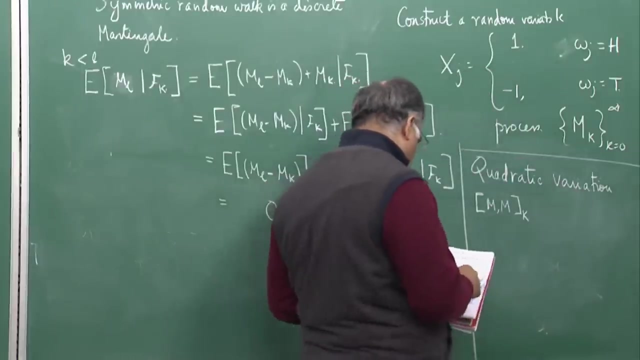 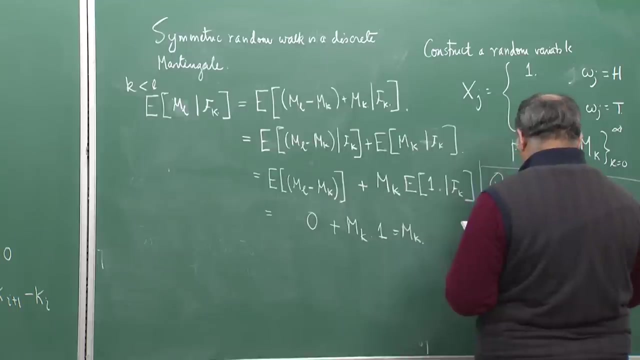 you just would not get any information. but take the square of the variation. It is like a mean square error type thing. So we again we take here and introduce the notion of a quadratic variation. So the quadratic variation is expressed in the following way: mmk is defined as summation. 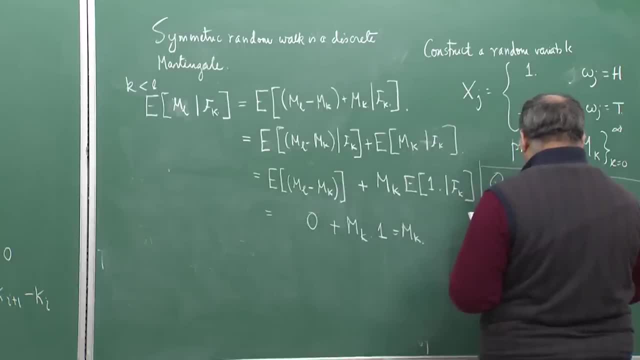 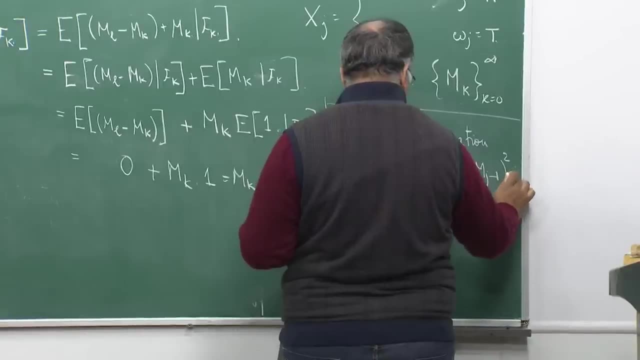 j equal to 1 to k mj minus m 0.. Ok, This is a pyramid equation. What is from this equation? it is written differently as this is a problem of k, Vegas And the 취 coefficient of k. this m? j minus 1 whole square is equal to: and this, if you look, m? j minus m j minus 1 whole square. 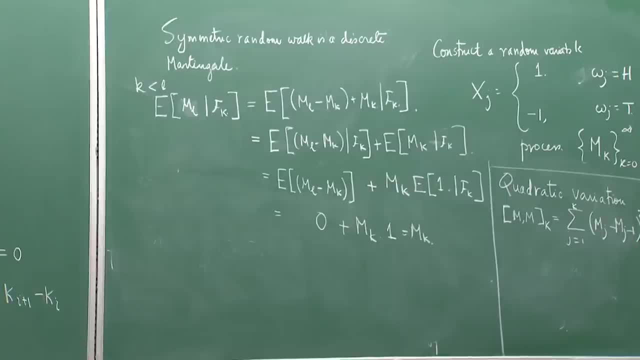 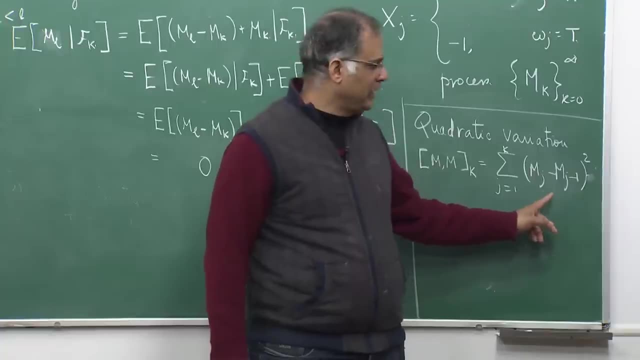 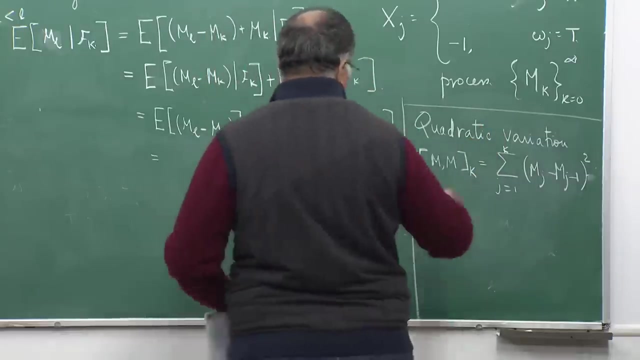 this value is always 1.. If you sum them up, what will be left here? x j would be left here the x j. if you take the difference between m j and m j minus 1, you will have the value x j left. x j is either plus 1 or minus 1.. So the squaring will always give you 1.. So 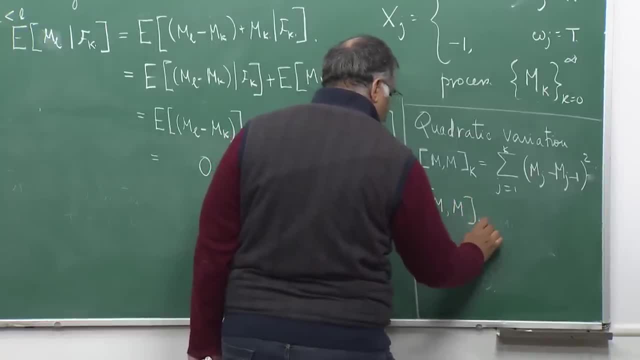 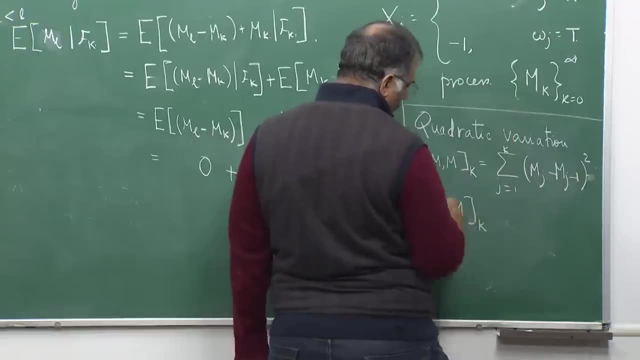 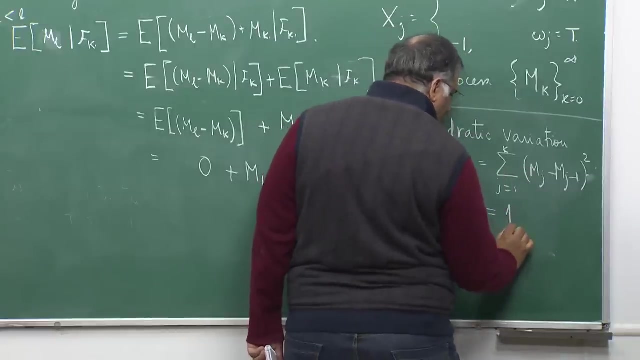 this expression of the square errors, basically, or the square changes around every path of a given sample. I can do that. take the changes, but it will, whatever be your path, independent of the path, it turns out to be k. If you do it up to the kth level, it turns out to be. 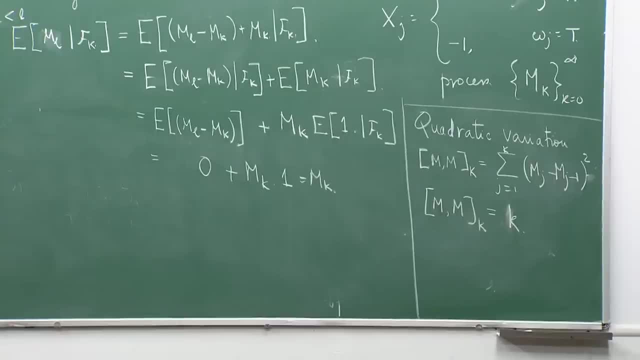 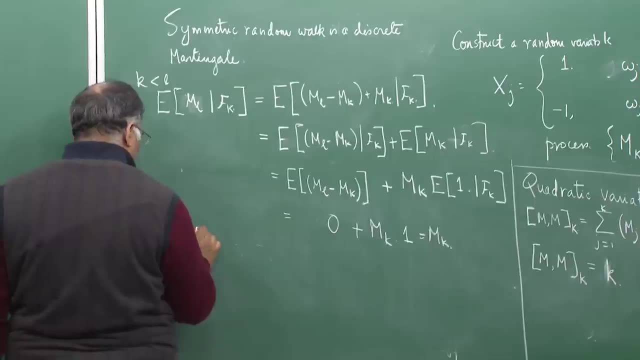 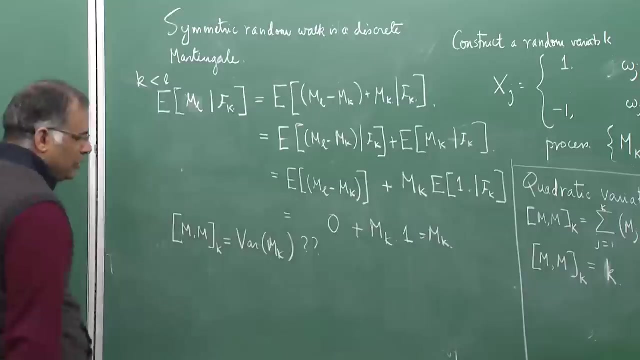 the k. independent of the path that you have taken, which is very interesting, it does not happen. for Suppose you want to So compute the variance. So m m k is actually variance of m of k. think about it how it possible. 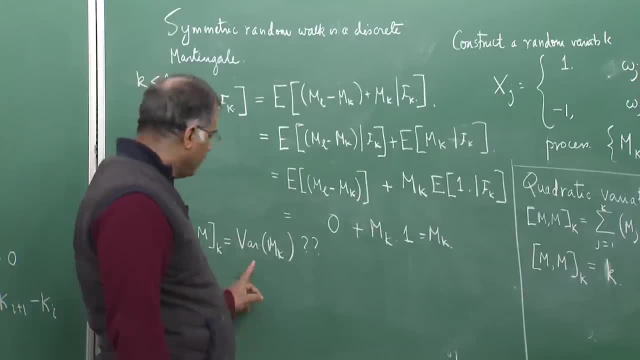 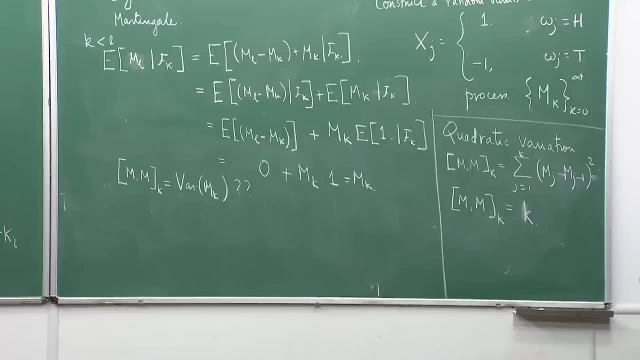 but you see, to compute this, I really do not need to bother about the path. but to take variance of m k, we are essentially averaging over all the paths. So this is a difference. Now, how do I, can I do something with this process? can I increase the jiggling of this? 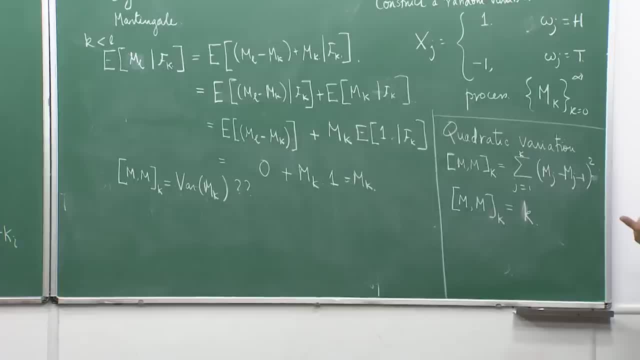 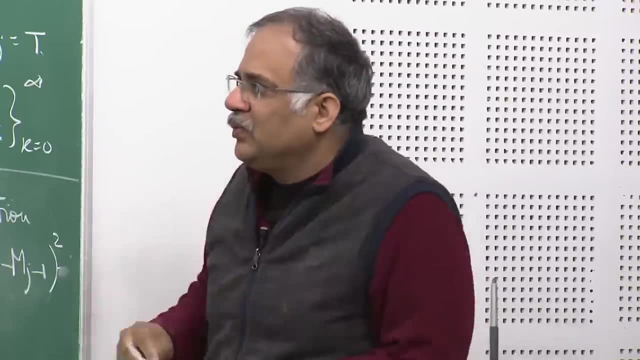 process of bit, this symmetric random walk of bit, and generate some sort of an approximation of a Brownian motion, generate this sort of zigzagging that we had just seen in the beginning when I had drawn the picture of the stock price. at this sort of zigzagging can we generate? 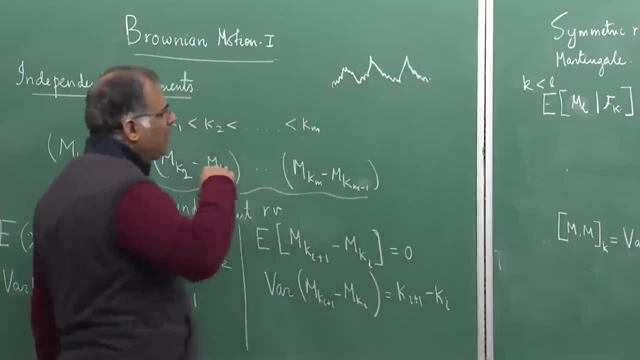 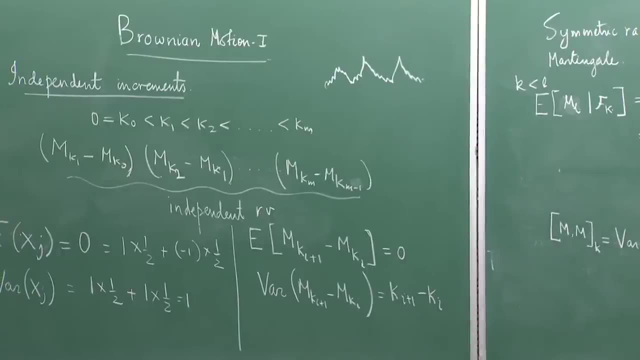 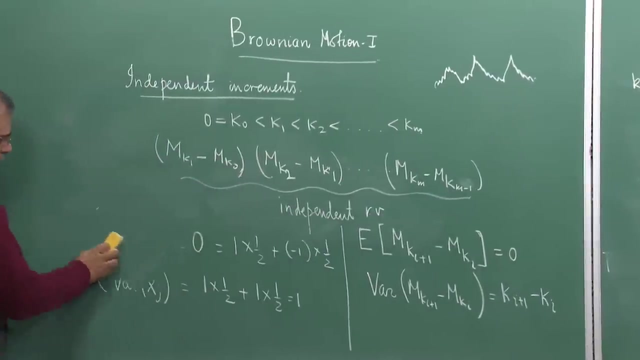 this sort of zigzagging. This sort of zigzagging can be generated by using the symmetric random walk, and that leads to what is called a scaled symmetric random walk. We will not go too much of details into it because that might, you know, take you off track and you might feel a little bit of discomfort. 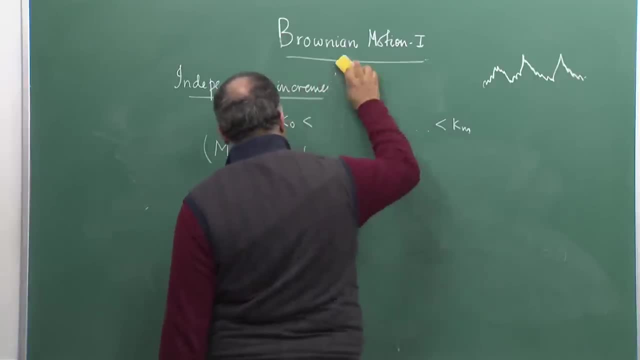 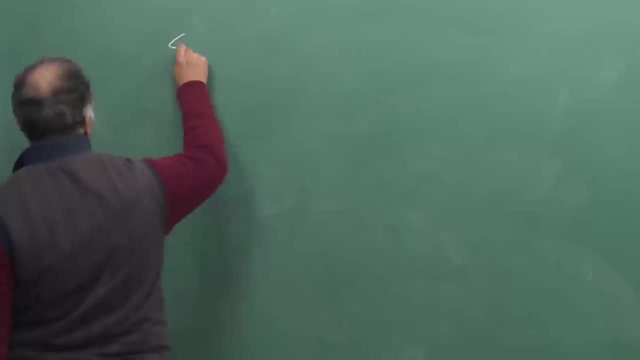 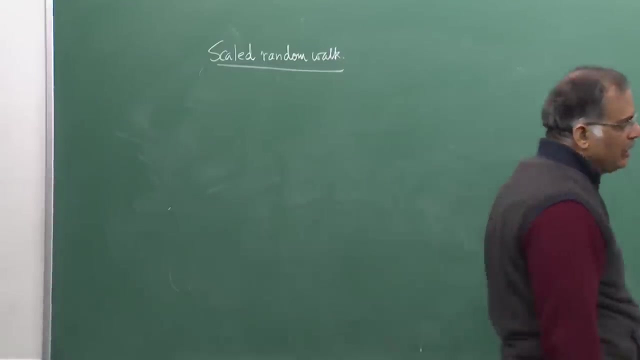 for those who are not So very comfortable with very complicated analysis. So what we are going to now show By this scaled random walk is that? what we are going to show by scaled random walk is that we can construct an nth level approximation for the Brownian motion. Let us construct. 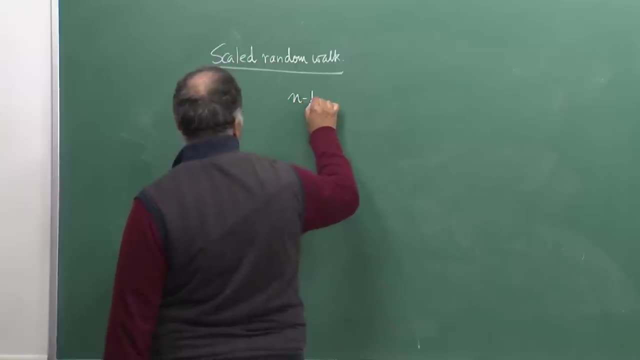 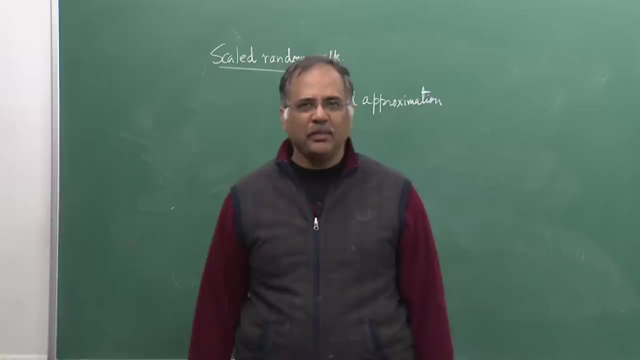 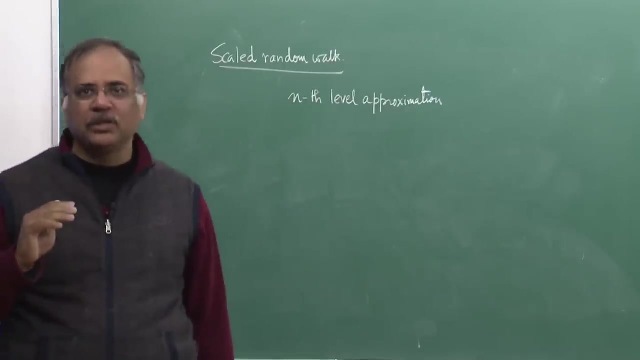 an nth level approximation. So if you are zigzagging by, say, plus 1 and minus 1, I might zigzag by 1 by 10th and minus 1 by 10th. So I will decrease my zigzagging steps but increases my time size, right? So 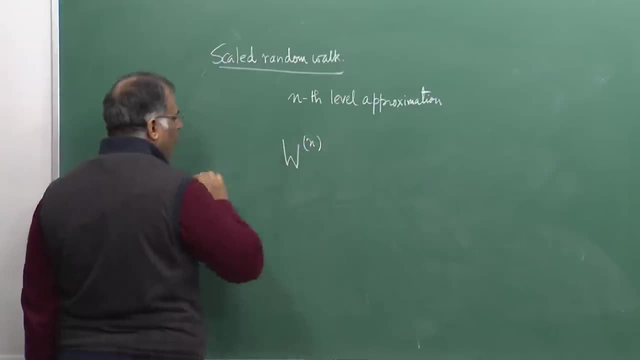 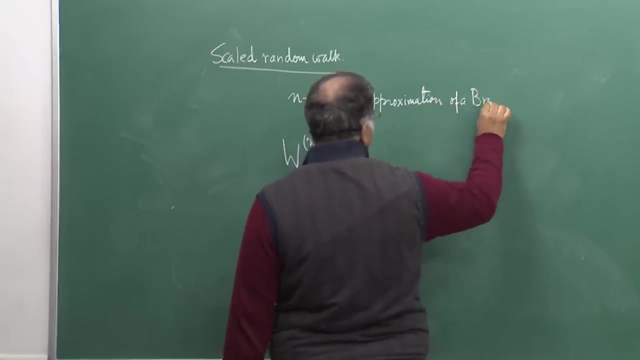 we construct the scaled symmetric random walk which is the nth level approximation of a Brownian motion. nth level approximation of a Brownian motion. So all these are stochastic processes. So this is a discrete stochastic process from which I am trying to go to a 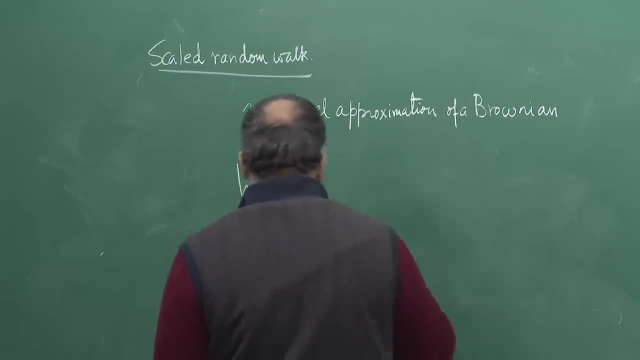 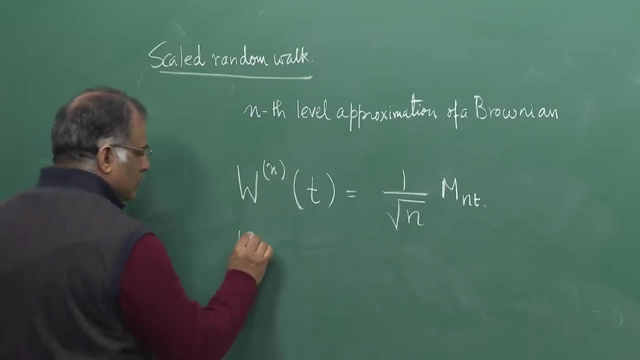 continuous stochastic process. I define it like this: See, if I do not have n t to be an integer, I cannot define this. So here my t is a t. say t between t starts from 0, and say it up to t, or even t goes to infinity. So basically, 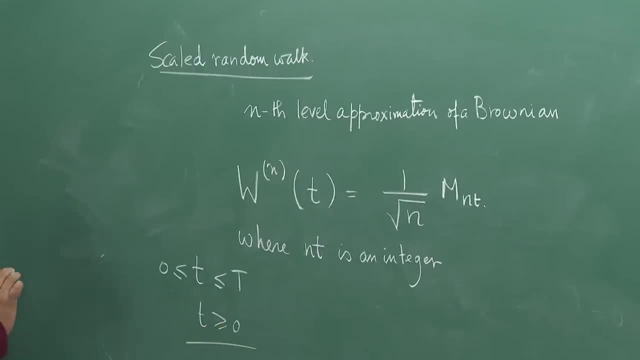 for me here this t is just greater than equal to 0. So I am So using the stochastic discrete thing, I am trying to construct a continuous stochastic process, but I have to be aware that if I really want to use it, So at the nth level approximation, this m 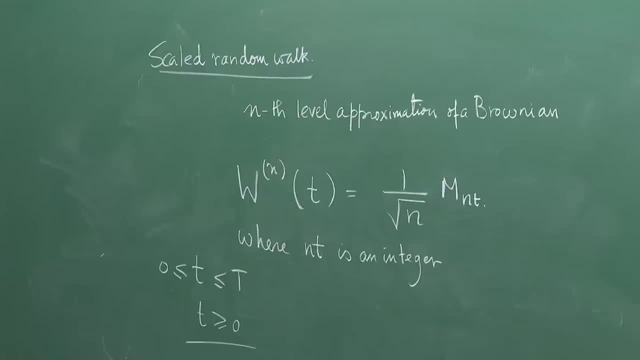 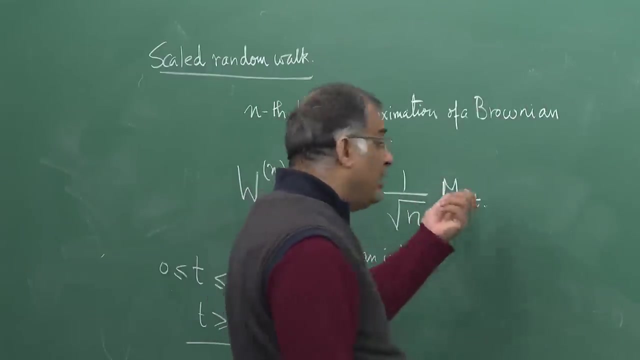 n? t has to be this. n? t has to be integer if I want to actually compute this. Otherwise, m is a discrete thing. it is computed only at integer points. you cannot compute it at non integer points. So what happens if it is not computed at, if n t does not turn out? 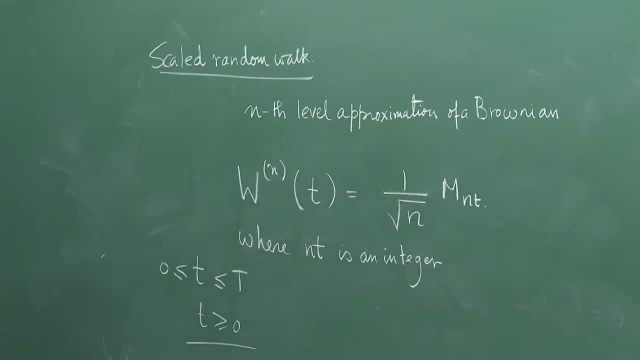 to be an integer. So basically, what you are considering for n very large at various time points, n? t would be a integer and you are actually computing at out of n? t. So if n? t is not an integer, take the t for which n? t is not an integer, then take some integer. 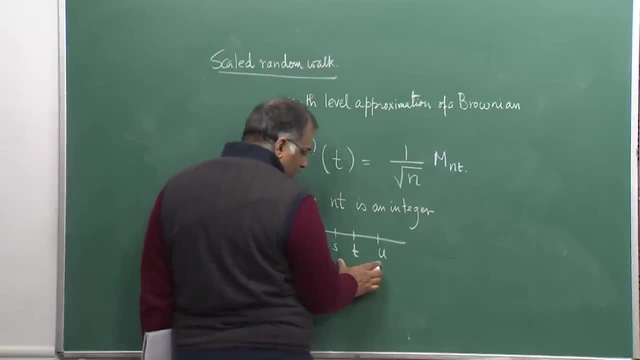 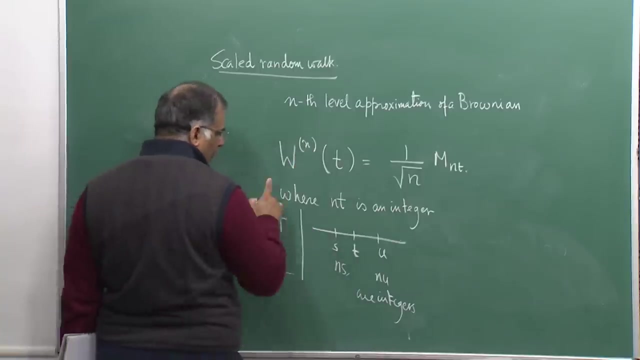 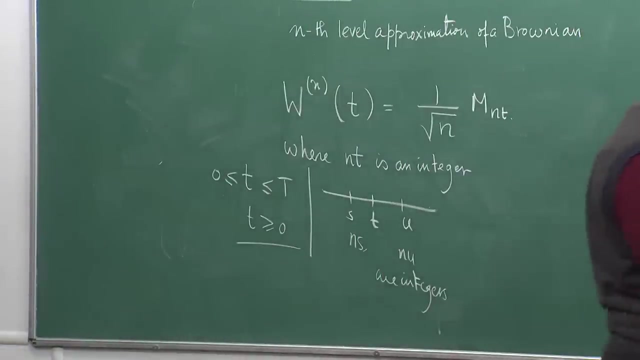 u and take some s which is nearest to t, such that n? s and n? u- these are integers- and then compute the value of w? n? u and w? n? s and then make an interpolation, linear interpolation, to approximate the value of w n? t. and that is how you can actually you do, you can generate. 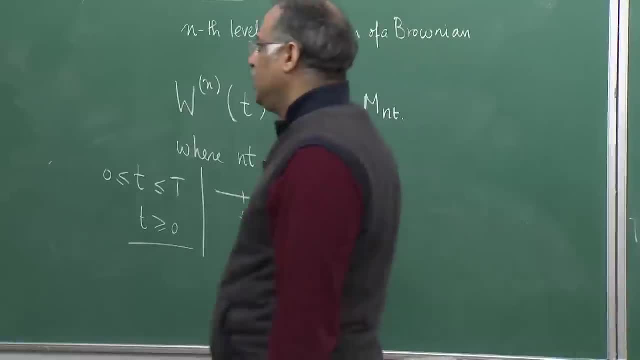 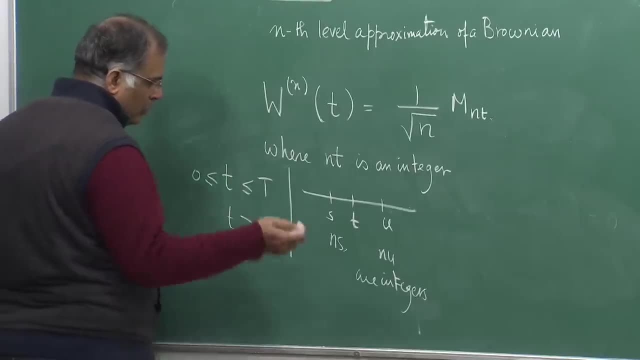 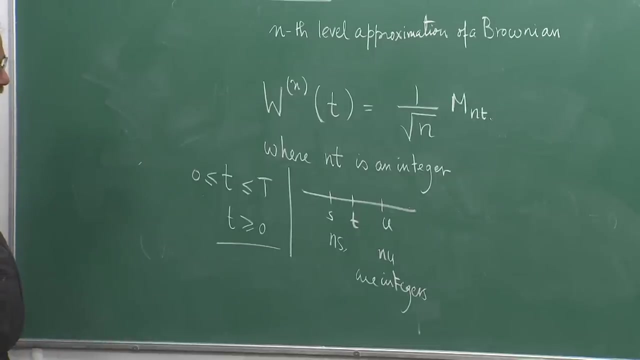 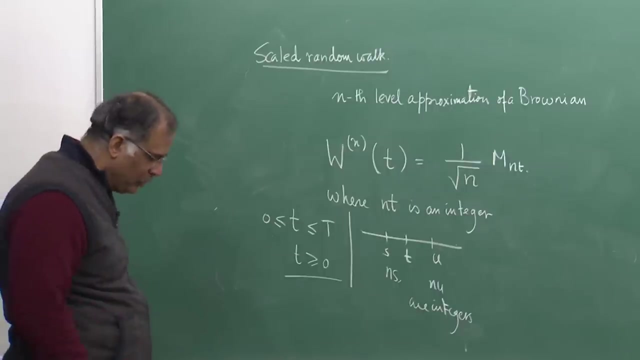 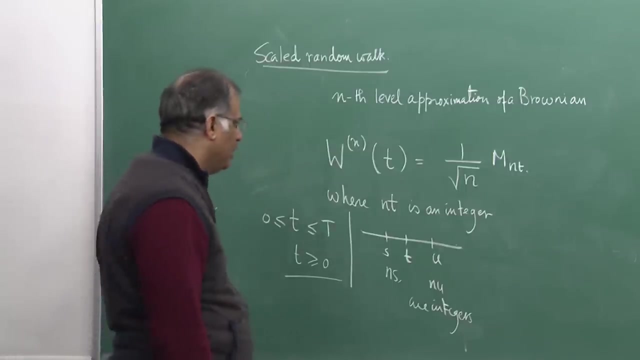 it in a machine by taking a samples. Say you can take a. you can take a sample of, say you can do the coin tossing four hundred times with one by tenth. you can toss a coin four hundred times with probability of half of going. you go one by tenth if it is h and you go minus one by tenth if it is tail. So 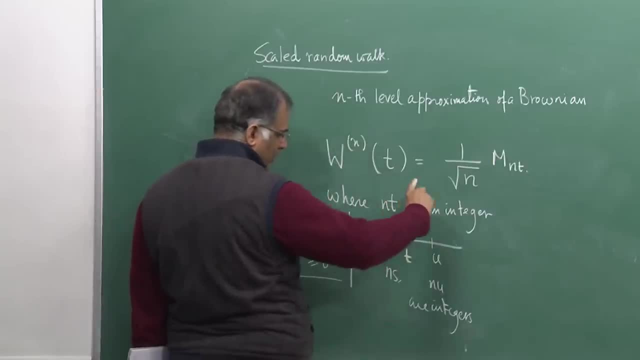 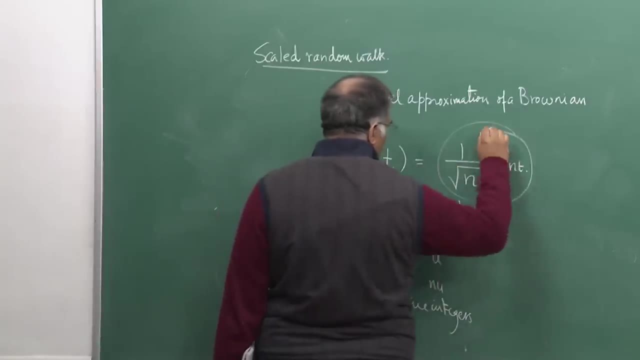 you decrease your movement, So you actually increase the zigzag by decreasing the movement, and at every time you have to observe that your m? n? t? n? t has to be an integer. Once you do that, you will find all the properties that you had of, for here is in here, provided.